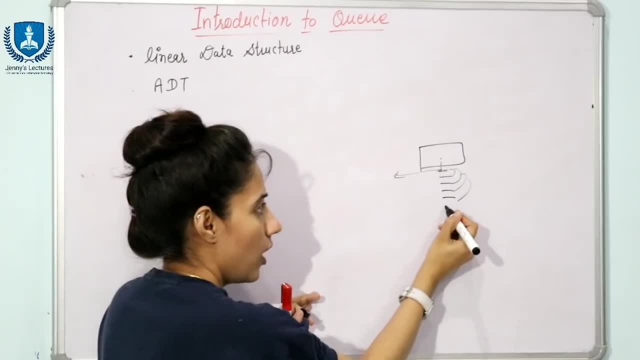 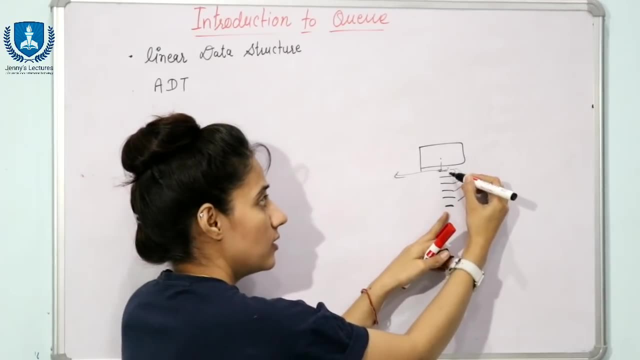 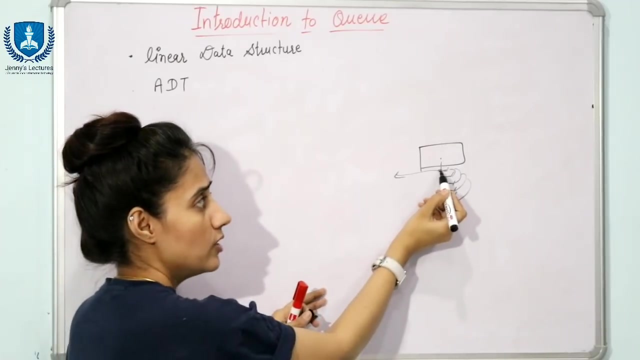 you, there are five persons and after that you reach there. so you have. you will have to stand at sixth position right and you will get ticket after the after you know the these five persons. fine, so here the simple is what first in, first out? or you can say: first come, first serve the person who is first in the. 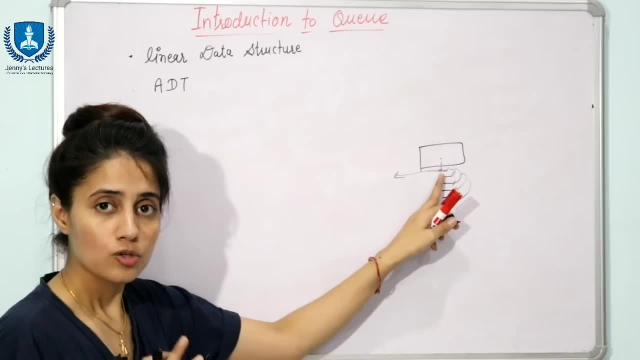 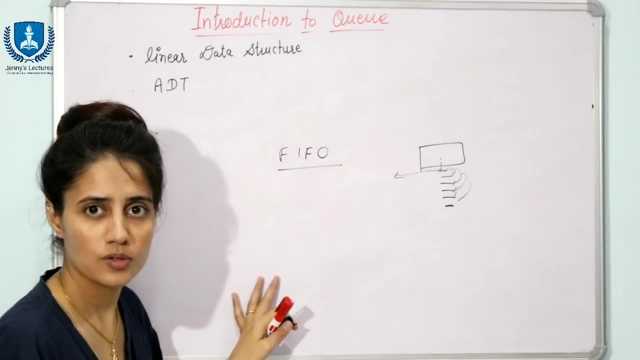 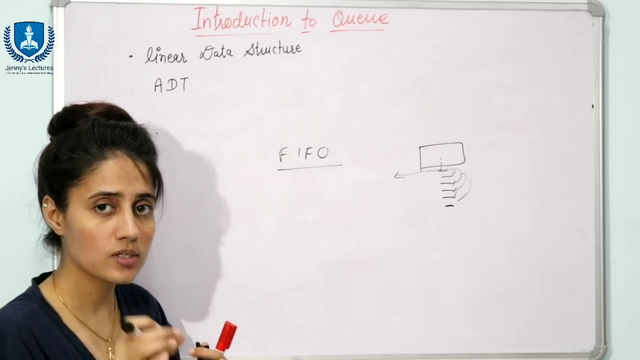 row will get the ticket first, right, so now in the queue. this funda is known as first in, first out, fifo. so q is basically what it is, a structure. you can say it is an ordered list as a stack. we have discussed. stack is an ordered list that follow the principle of lifo: last in, first out. 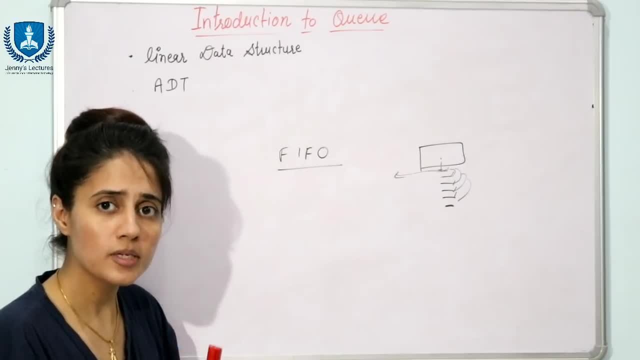 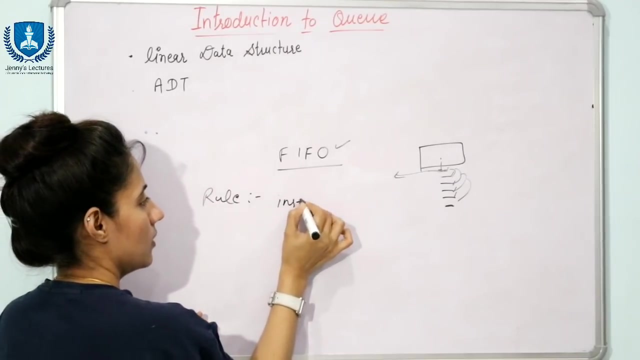 q is in collection or q is an ordered list which follow what principle? first in, first out. right now, what is that principle? see, you can say q is a structure that is going to follow some restrictions on insertion and deletion operation, fine. or that is going to follow a rule that is going to follow a principle. and what is that rule? insertion and. 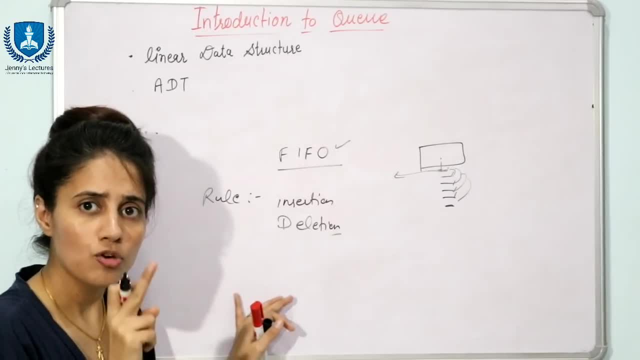 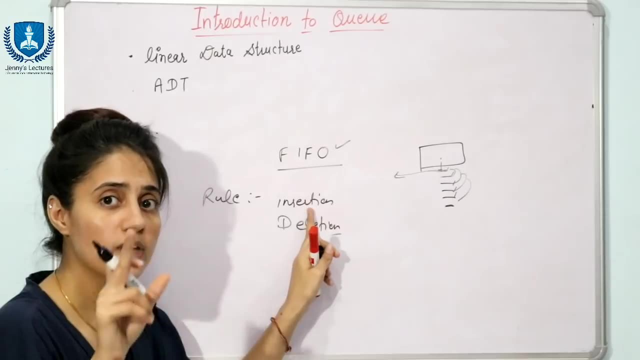 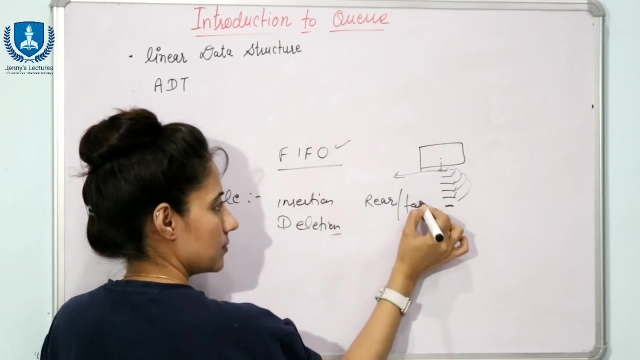 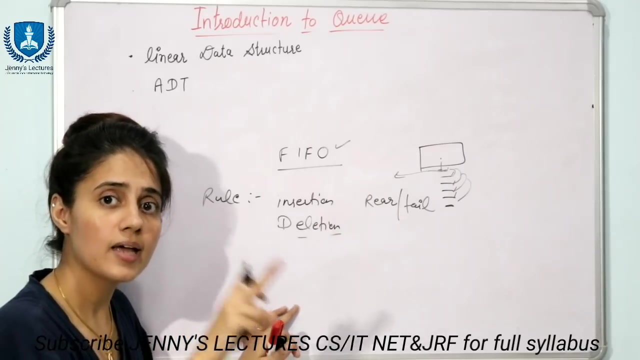 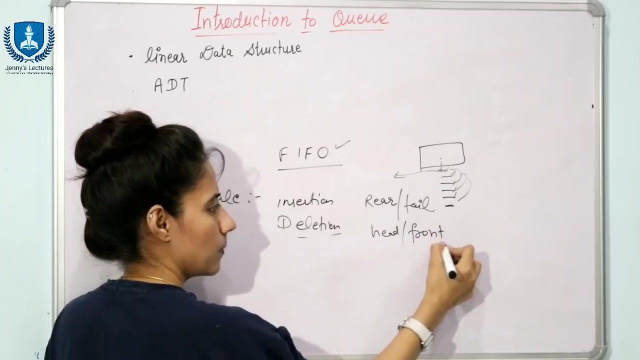 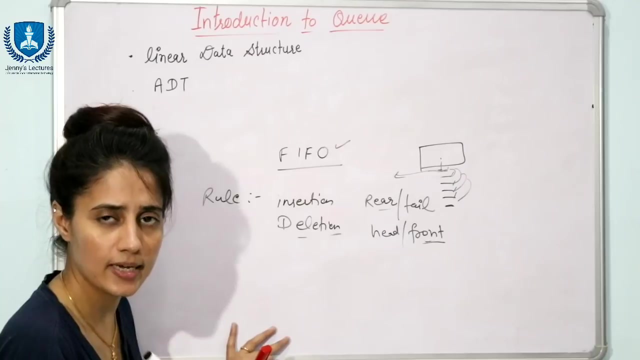 deletion and deletion in case of q, insertion would be performed from one end, right, and the name of that end. that end is known as rear or tail right, and deletion would be performed from another end and that end is known as head. or you can say front right in q. if you say more technically, then we will use rear and front, not head and tail. 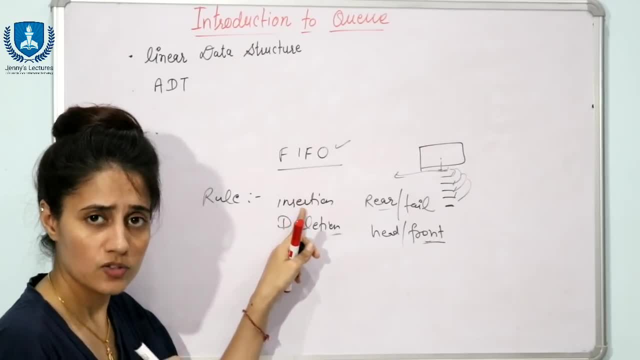 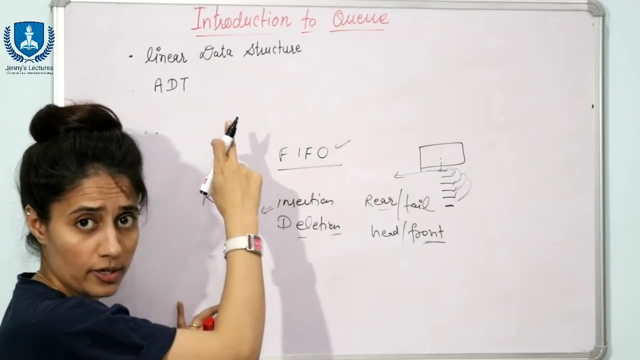 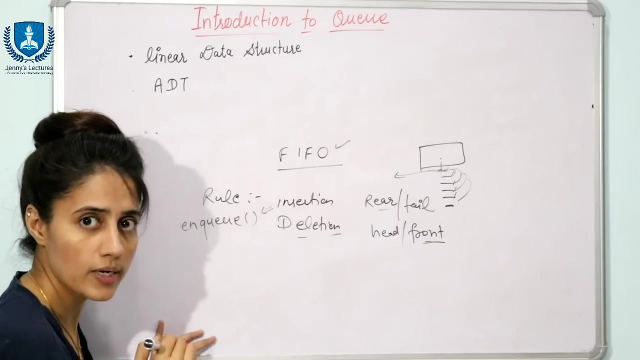 and rather than insertion. insertion means adding a data in the q- fine, so the technical name in the in, in this, in the context of q, it is known as nq- right and deletion is known as dq. fine, and in stack, this insertion and deletion is known as. 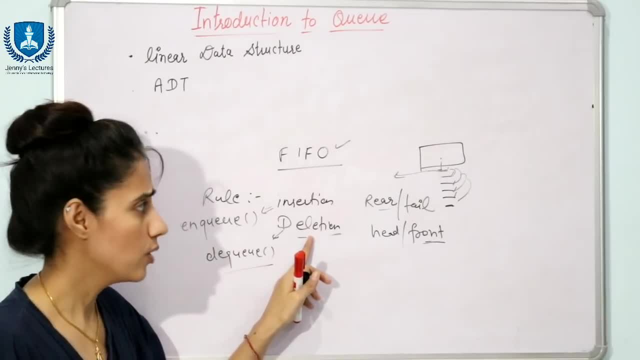 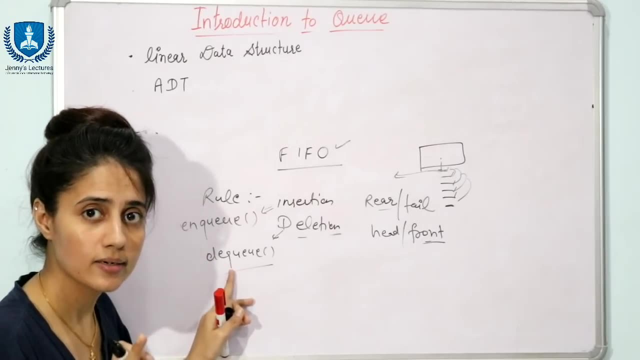 push and pop. fine, so nq operations would be performed from one end and dq operation would be performed from another end. right? so we will see the logical representation of q. if you logically represent the q, and dq operations would be performed from one end and dq operations would. 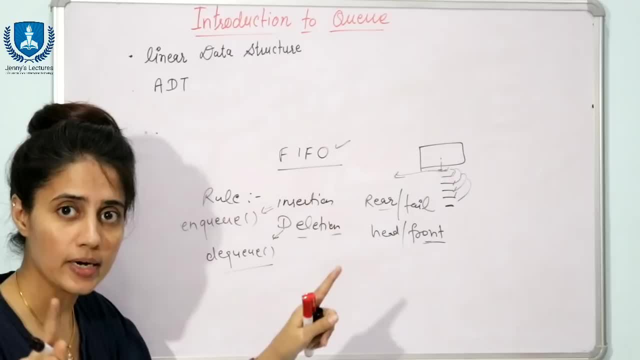 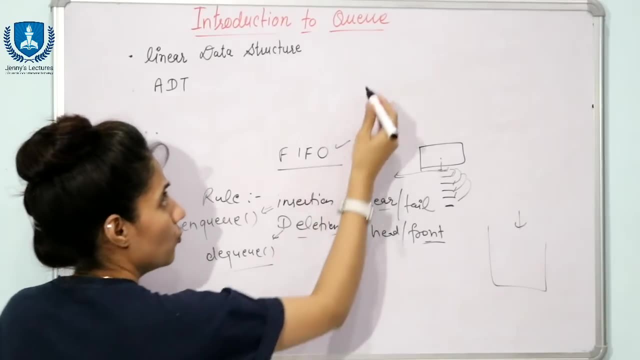 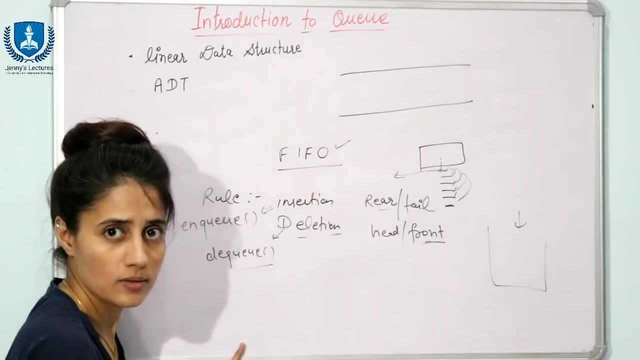 be performed from another end. it will have two ends, two open end right. in stack we have only one end, one open end right, and q would be represented something like this: it is having two end. one is this one? is this right? suppose i am taking this end is rear. 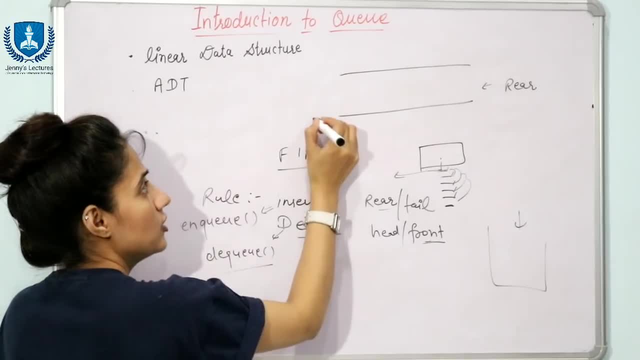 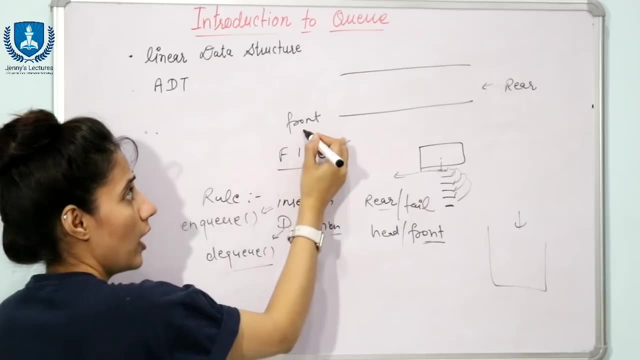 right, and this is what front front. obviously, when you are going to do the work of the vertical axis, you are not going to have two ends, right, because if you are going to have two ends to implement this queue, you will have to take front and rear, two variables. right, that is must. 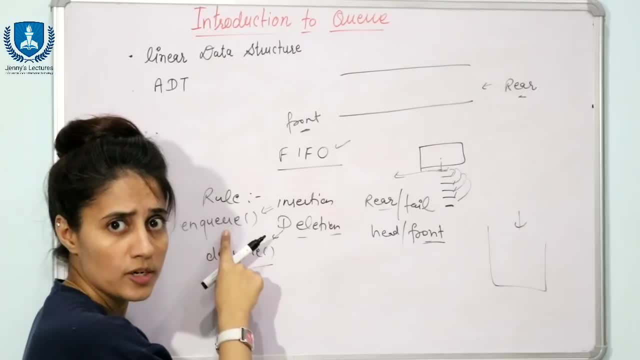 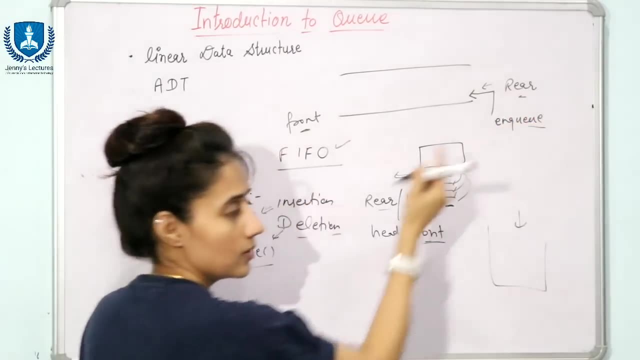 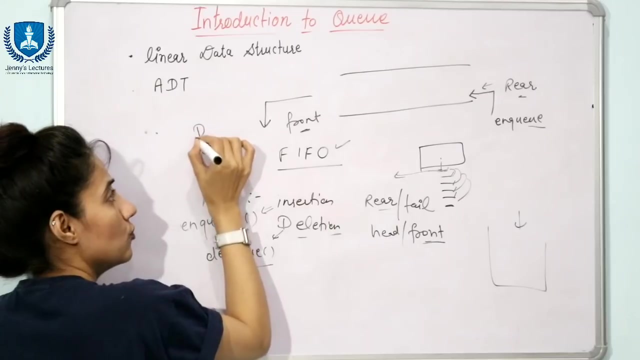 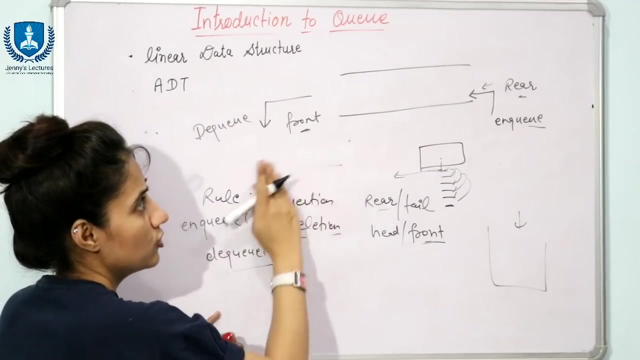 so insertion or you can see, nq operation would be performed from rear. from here we can insert data in the queue and if you want to delete data from the queue, it means from the front, we can dq, we can delete data, right. so this is what logical representation of a queue. fine, suppose nq i have. 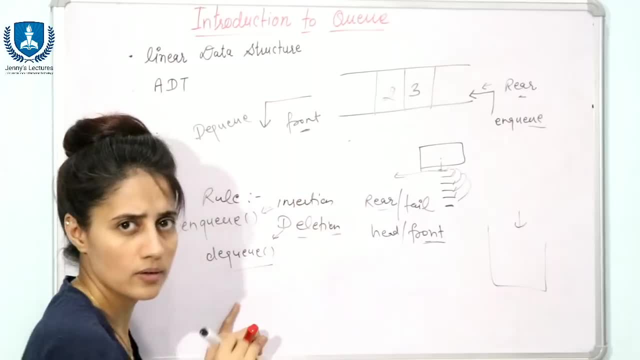 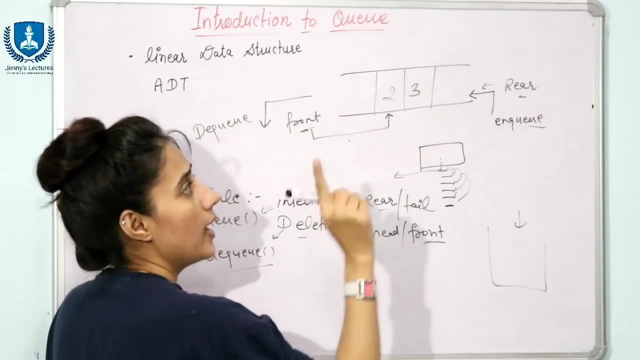 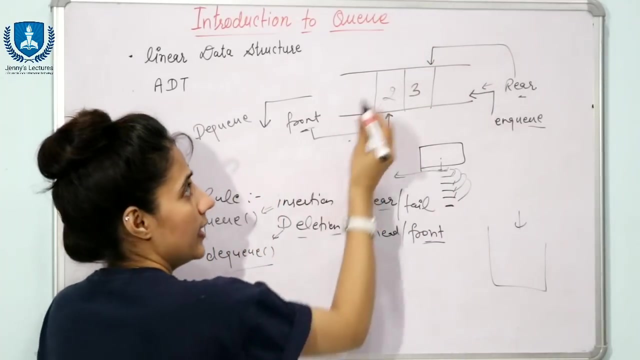 right now, two elements, two and three at some point of time, right. so at that time this front variable would be pointing to here and the rear variable would be pointing to here. right, and the index is suppose right and the index is suppose right and the index is suppose. 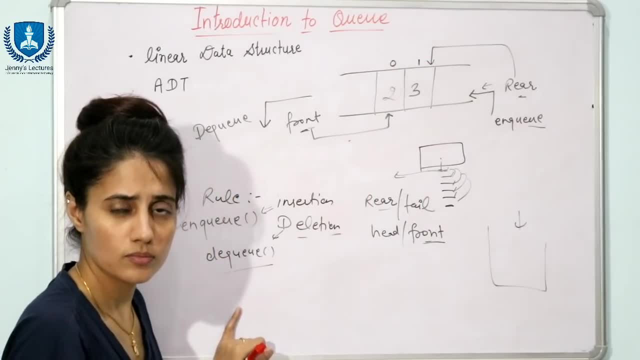 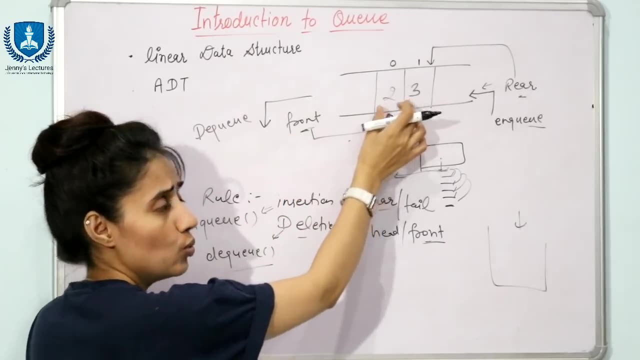 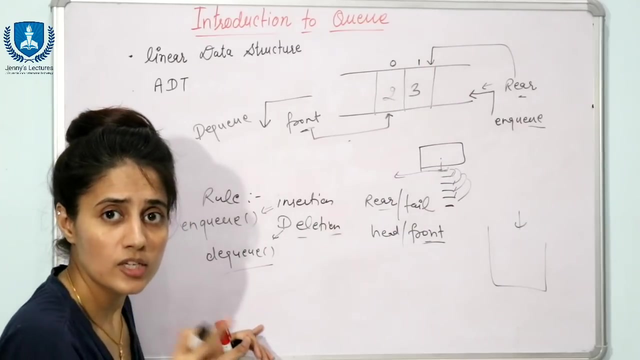 0 and 1. now, at some point of time we are suppose we are implementing this queue using array and at some point of point of time we have only two elements in the that queue and index is 0 and 1. so front is 0 and rear is 1. now, in this case, if you want to insert third element from where we 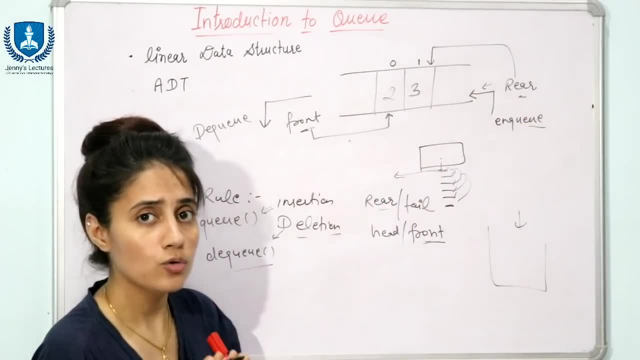 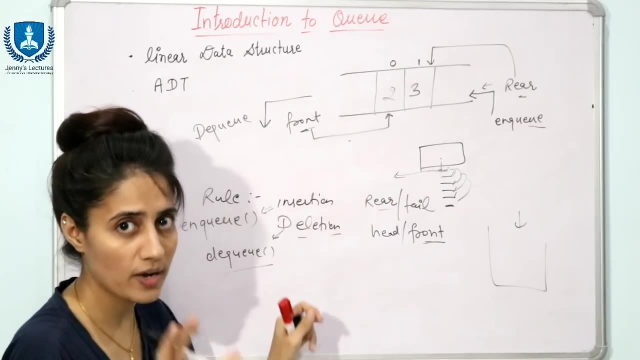 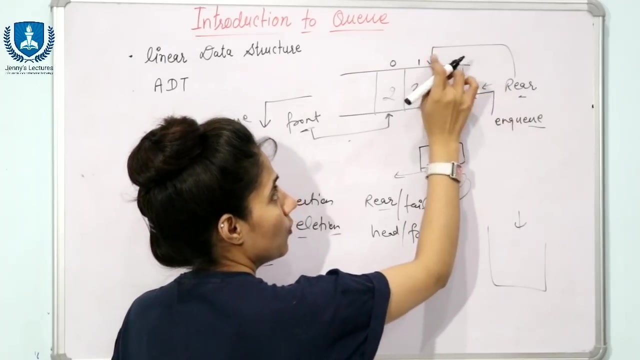 can insert from this end, only so what you need to do. if suppose the size of this queue we have taken 5, we can insert 5 element. the capacity is 5, right, so now, first of all, you will increment this rear, right, so now, rear plus. plus, that is rear would be pointing to this node. and now you 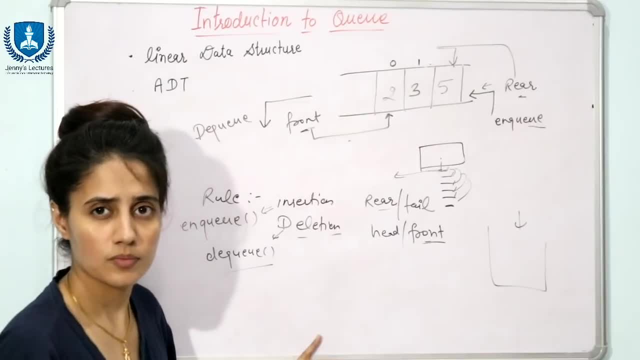 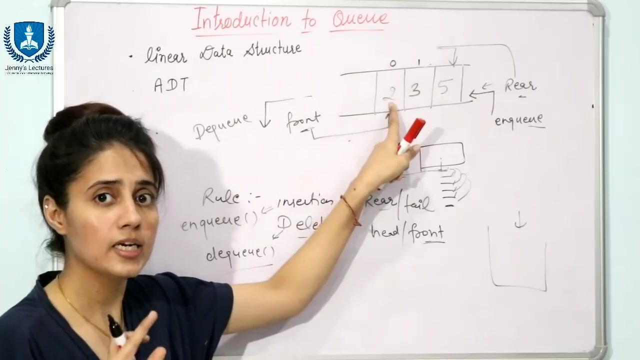 can insert another data. suppose i have inserted 5, right, and if you want to delete, then from here only you can delete, right. so first in, first out, firstly we have inserted 2 and that is the first element you can delete. if suppose you want to delete this 5, you cannot directly delete. 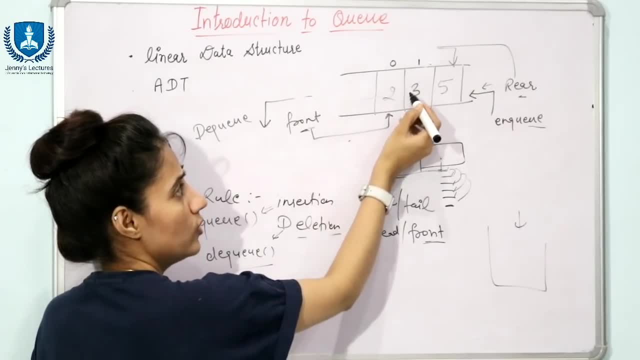 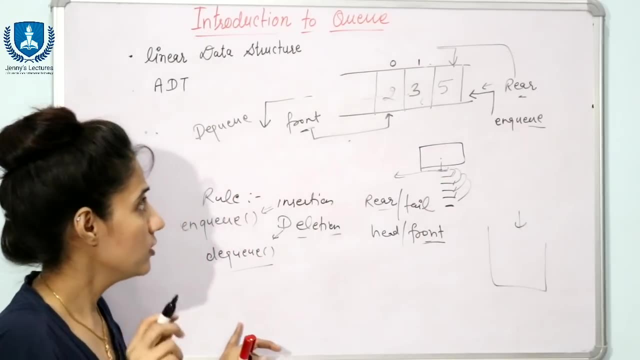 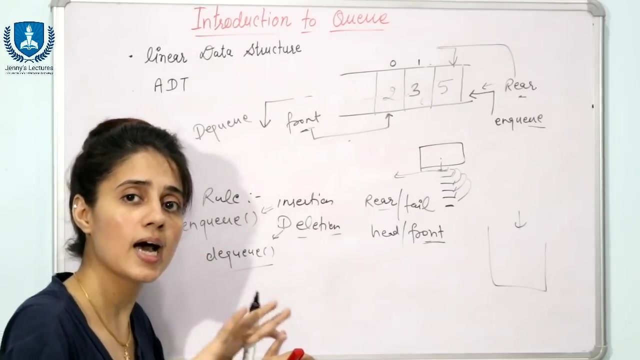 this 5. first of all, you will have to delete this 2 from the queue, then 3 from the queue. after that, only you can delete this 5, right? so it is. that is why it is known as it will follow FIFO principle: first in, first out, or you can say last in, last out, last in, last out, somewhere it is. 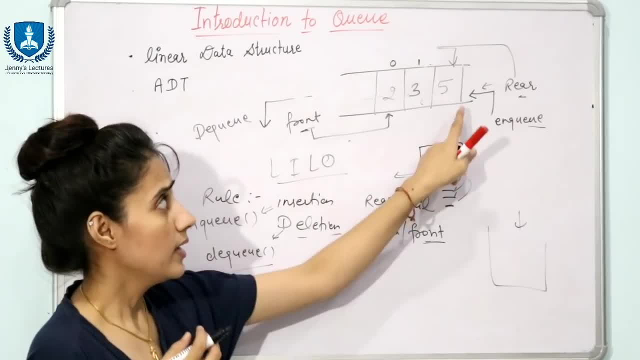 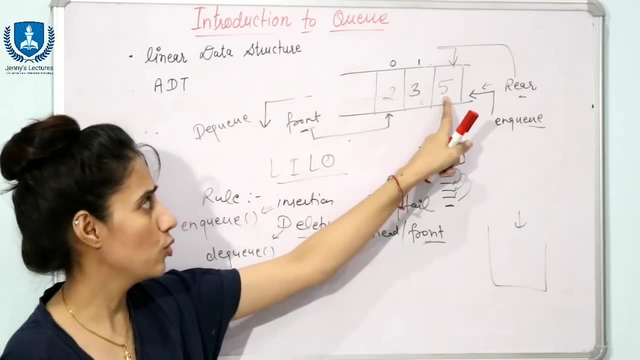 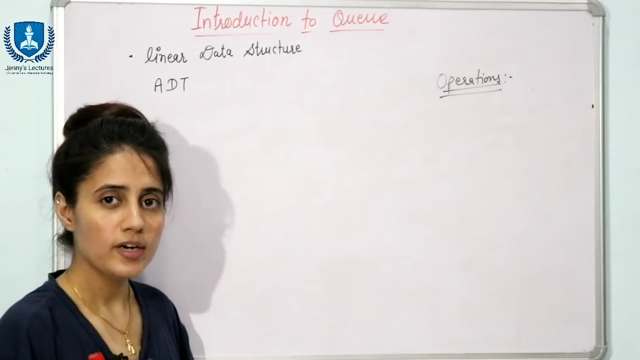 also written like this: that is same thing. last integer that is in queued in this queue is 5, and that would be the last element you can remove. so last in, last out, this is queue. so now we will see some operation that can be performed on a queue. so you can define queue as it is a ordered list, or you can say it: 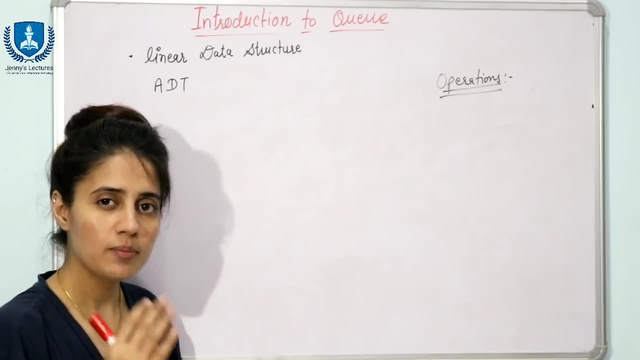 is a collection in which insertion can be performed from one end, that is, from rear end, and deletion can be performed from another end, that is, from front end of the queue. fine, and it is going to follow. it is a structure you can say that is going to follow the FIFO rules. that is first in, first out, right. so now we will see some. 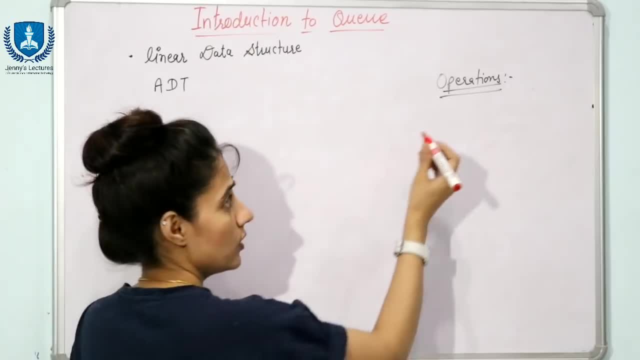 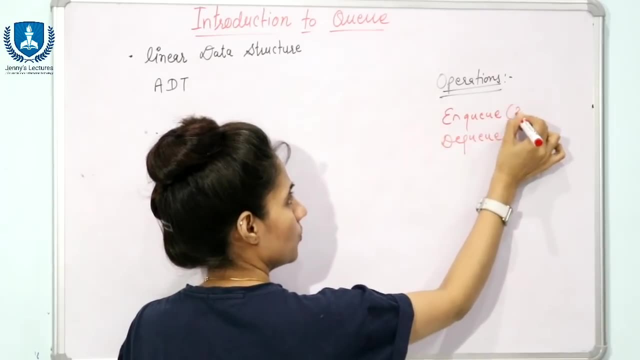 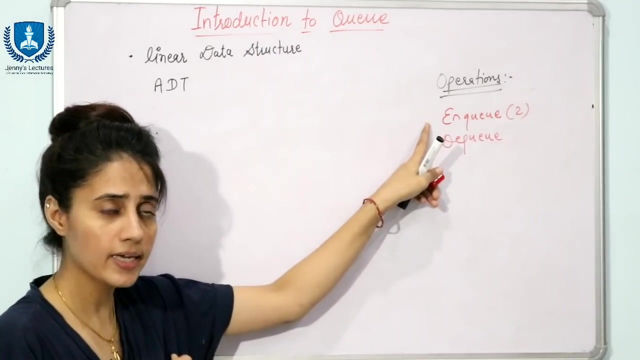 operation that can be performed on queue. so two operation we have discussed. that is first is NQ and that is second is DQ. right, these are two fundamental operations: NQ and DQ. NQ means inserting or adding a data in the queue and DQ means inserting or adding a data in the queue. 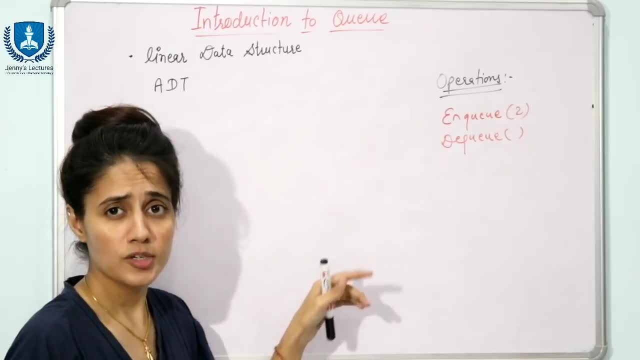 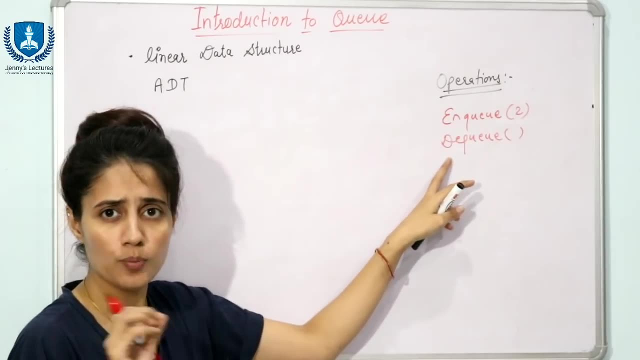 DQ means deleting a data from the queue. see here in NQ I am passing two as an argument because I want to suppose I want to insert two in the queue. then I can pass this in the NQ. in DQ no need to pass anything because always the element would be DQ from the front. so the element which is at the 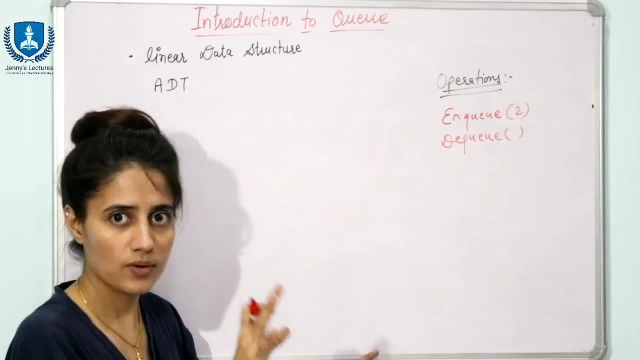 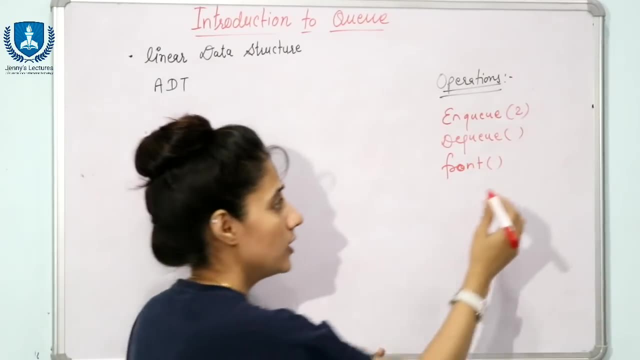 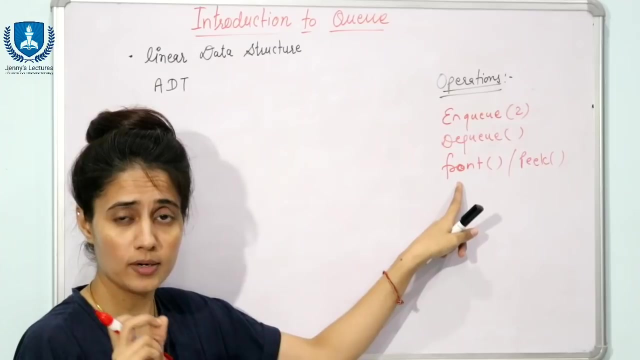 front index of the queue. that would be deleted right, so no need to pass anything. third may be front, or you can say peak in stack in stack it was top. it means the motto of this operation is what it is going to tell you. what does the element at the front of the queue? 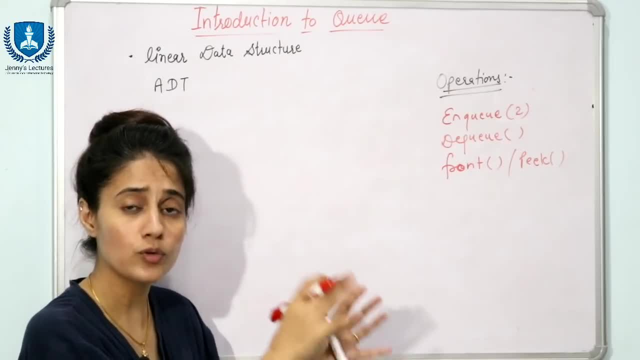 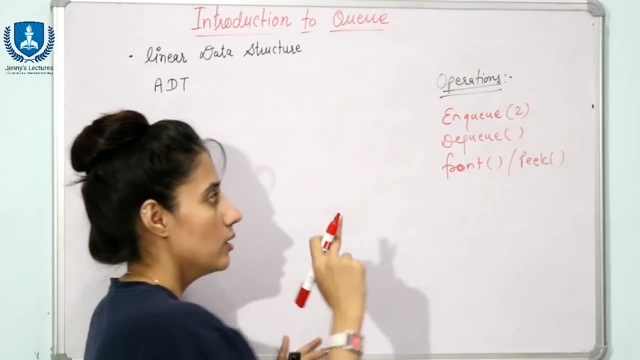 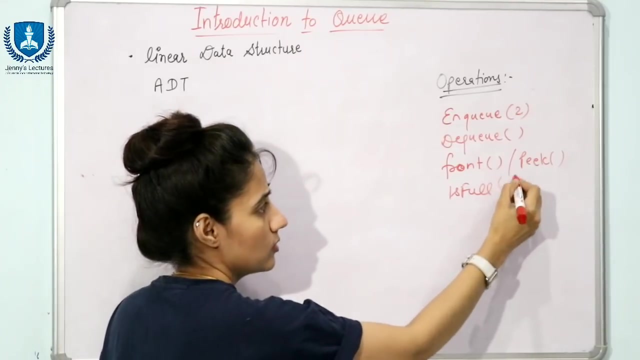 right, we will see what is the element at the front of the queue without removing that element from the queue or without DQing that element from the queue right now. isq You can check by- Is Full function. it is, it will return true. 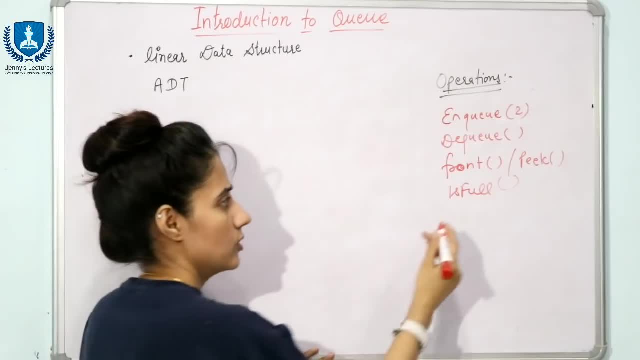 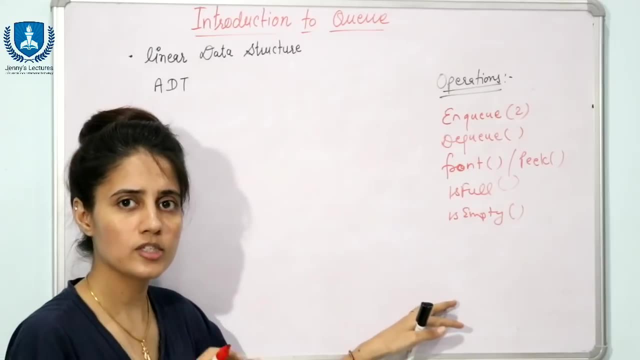 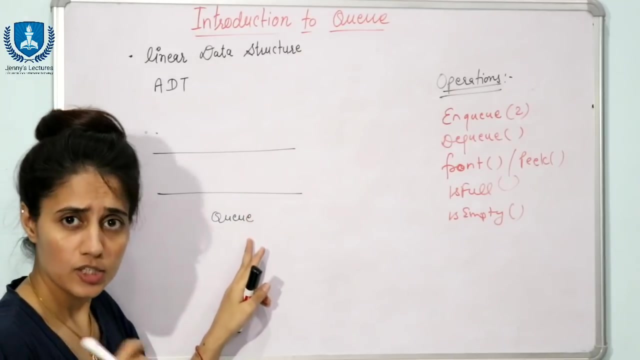 If the cue is full, it otherwise it will return false, is empty. same we have discussed in stack: if the q is empty, then it would return true, otherwise it would return false. right now, see the logical representation of q. so this is the logical representation of q. fine, any end. you can take front or 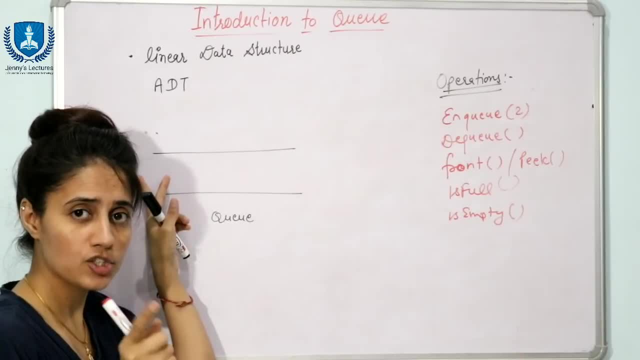 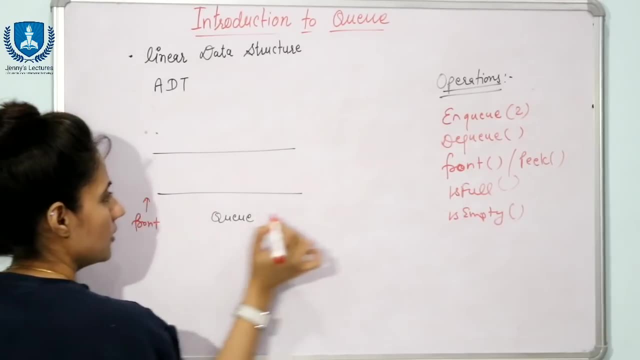 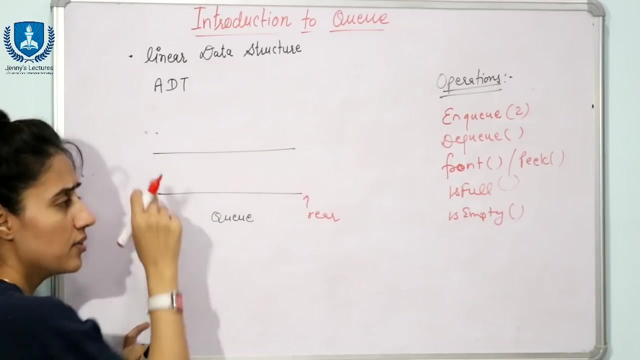 rear. but you have to take care of that thing. deletion from front and insertion from rear, right. so here i am taking, this is what front and this is what rear i will insert always from here, delete from here. you can take front this side, rear this side, as you wish, but insertion. 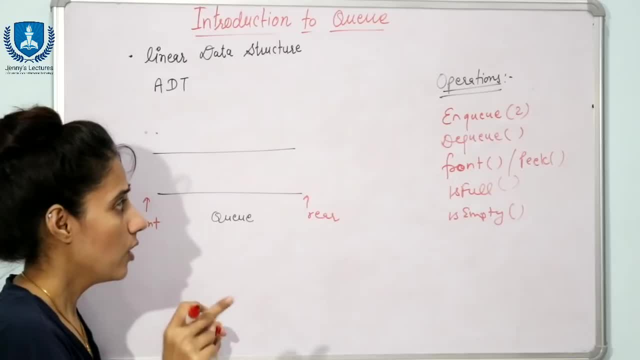 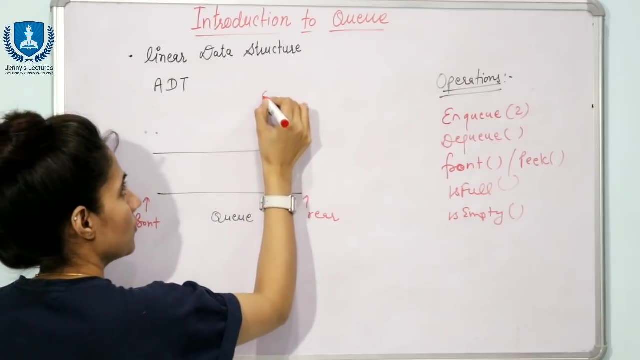 and deletion would be, according to the rule, only fine. now, if you want to insert some data here, obviously you need to specify the size of this q. suppose the capacity of q is 5, you can say: size i am taking is 5. how we will take the size 5? 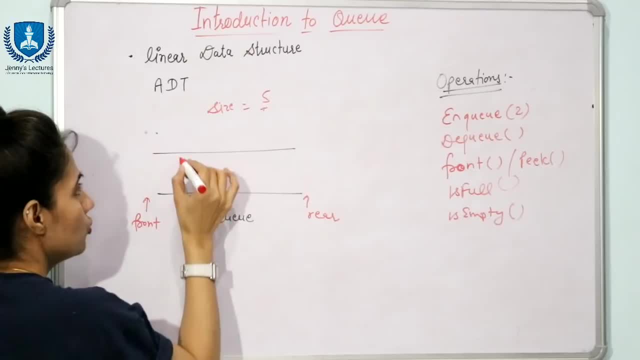 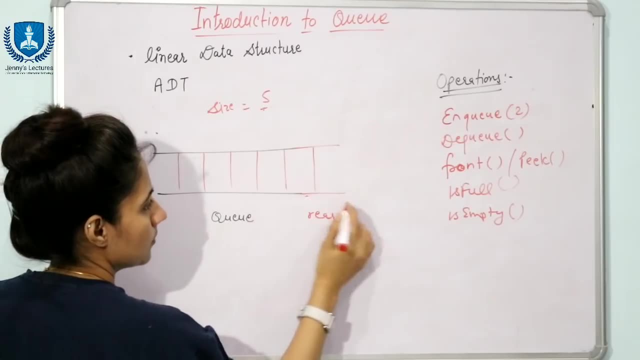 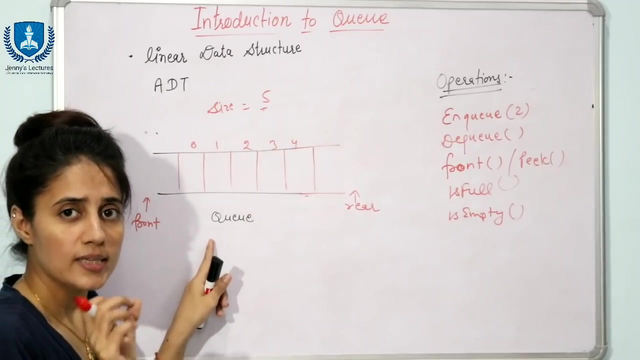 how we will implement this q, that thing we will discuss in next video. so it means i can insert 5 element in this q right. here i have this end and index is 0, 1, 2, 3 and 4, so initially there is nothing in the q right. in that case, what we will do, both front front end- this: 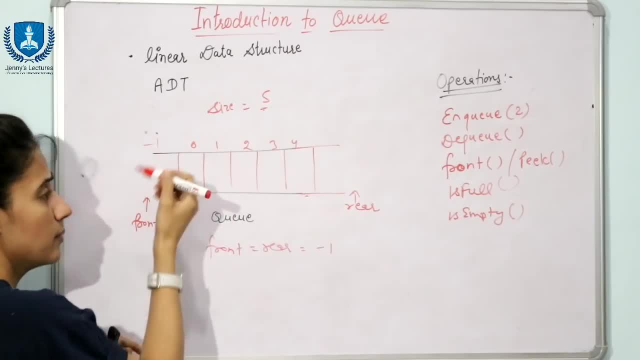 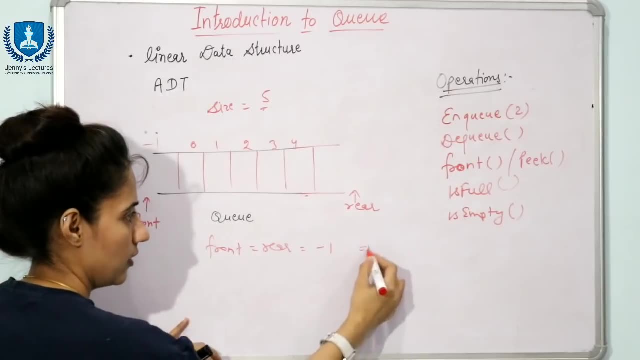 rear would point to minus 1. hypothetically, we assume that there is a minus 1 index and these are pointing to minus 4.. 1, it means q is empty. right, that is the signal. if this is minus 1, it means q is empty. now i want to. 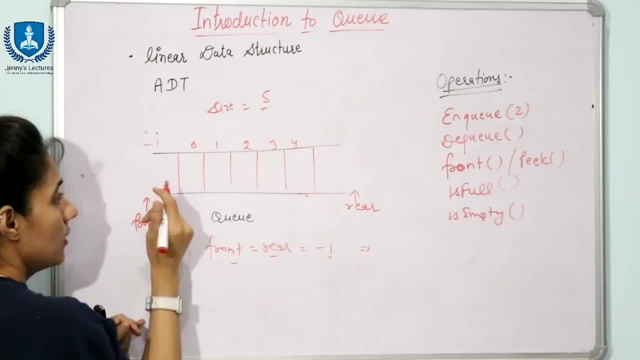 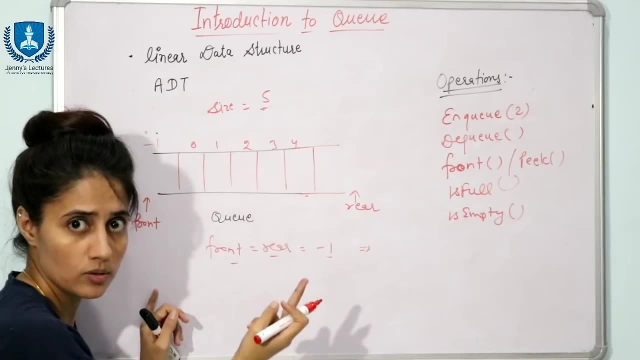 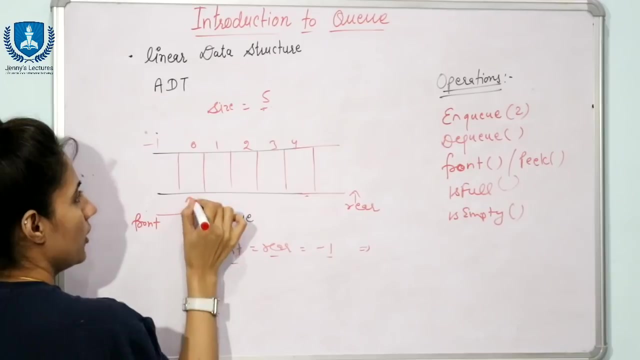 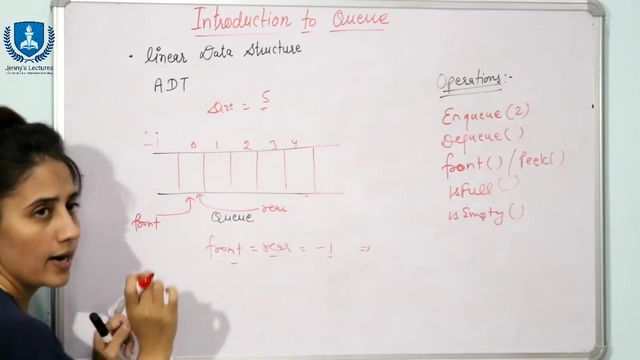 enqueue 2. now what would happen? see, front is minus 1, rear is also minus 1. obviously we will increase front and rear both. so front plus plus and rear plus plus also right. so now front is also pointing to here and at this point of time rear is also pointing to here at 0, and now we can insert here: 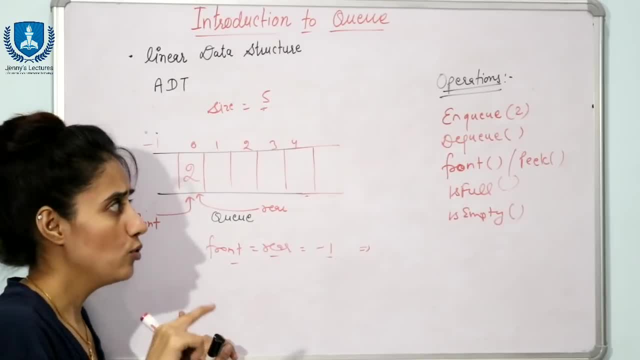 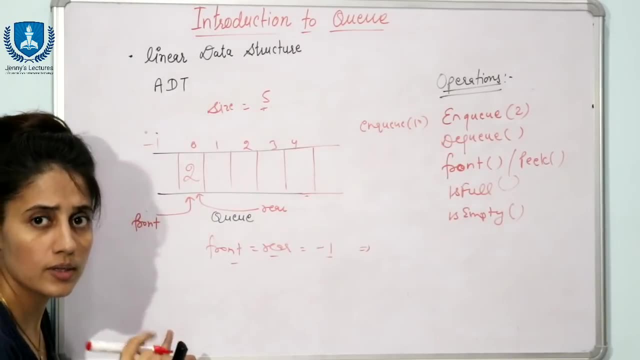 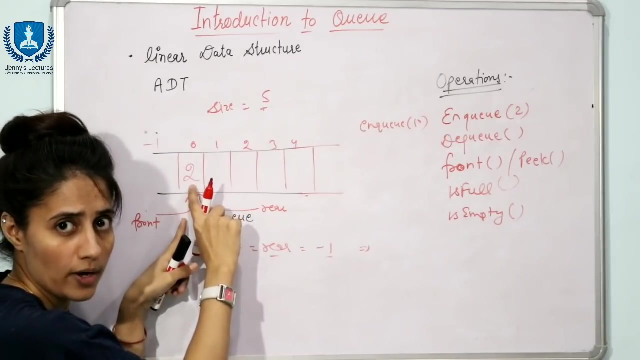 too right now. suppose again, i want to enqueue 3, i have called again function enqueue. and suppose 10, i want to insert. in that case what will happen? see front will always point to this node, the front 1, the front element. we will not move this. 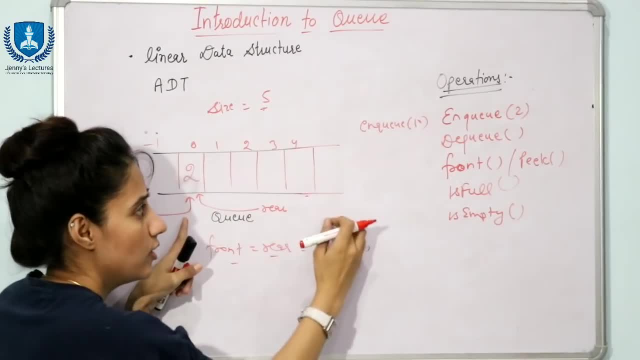 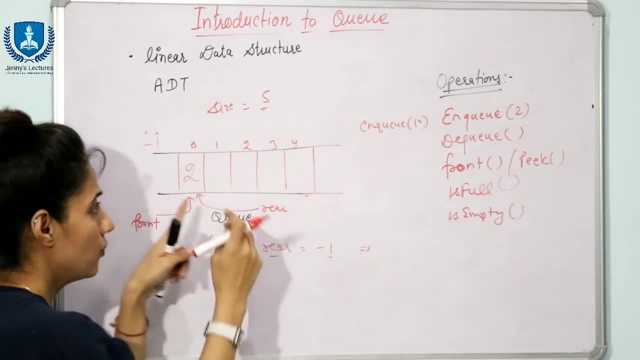 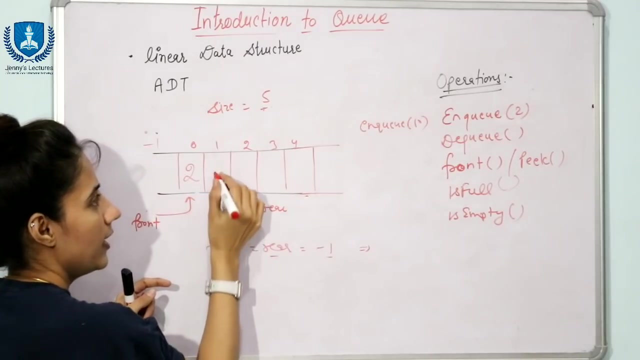 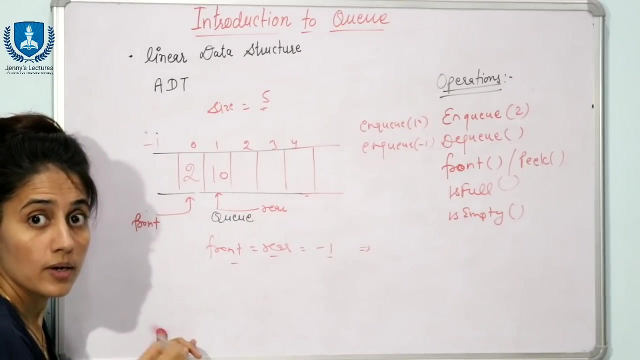 front for inserting the data. inserting would be always from the rear part. so the rear variable we are going to move. so first of all we will increase the rear. rear plus plus means now rear is pointing to here and now here i can insert 10 again. suppose i am calling enqueue minus 1, again what we will. 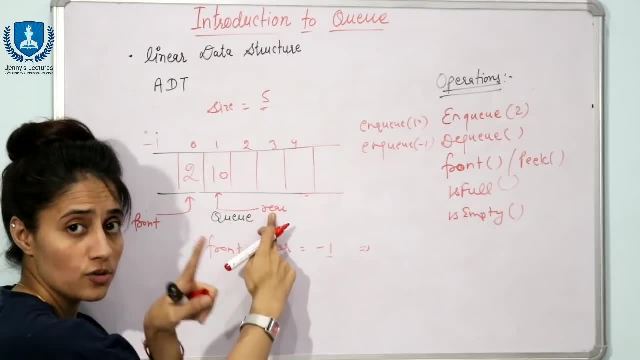 not touch this front. we will move this rear insertion from back to front. so we will not touch this front. we will move this rear insertion from back to front. so in this scenario we are going to rear. only that thing you have to take care: rear plus plus means rear would point here and now. 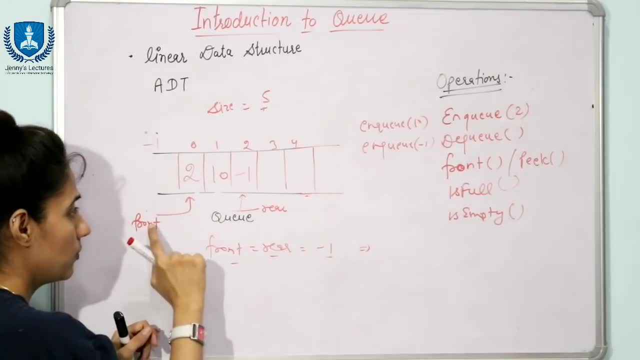 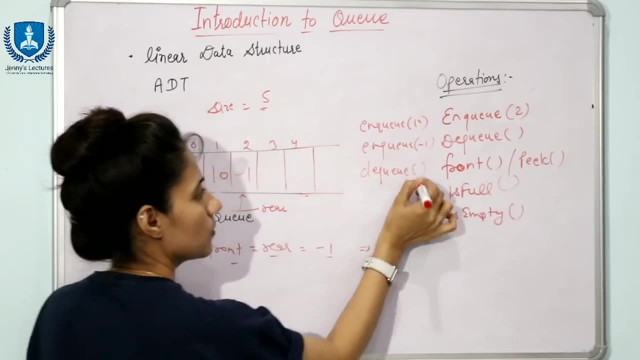 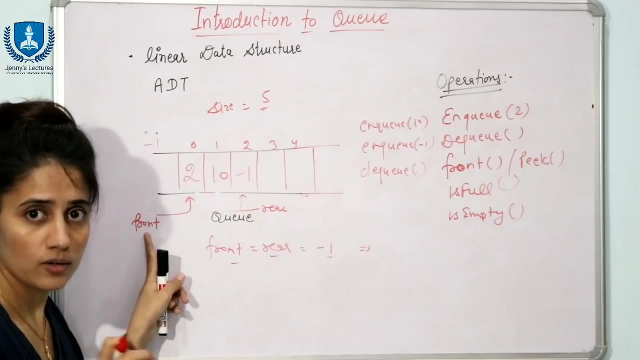 here i can insert minus one. see, at this point of time front is zero and rear is now two. right now, suppose i am calling dq function. no need to pass anything, because always the data would be deleted from front. now you can touch this front. now we will not touch this rear in dq, we will touch this. 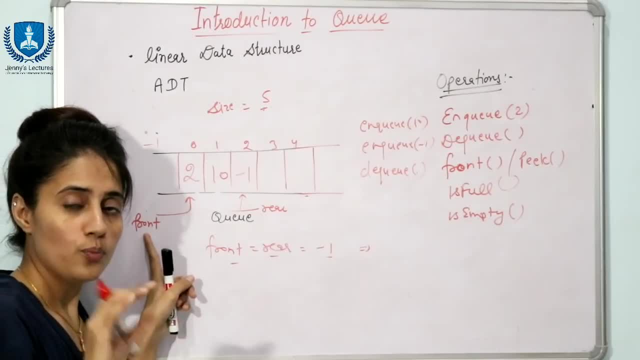 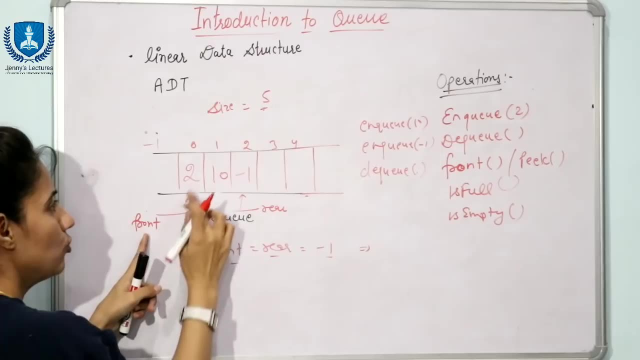 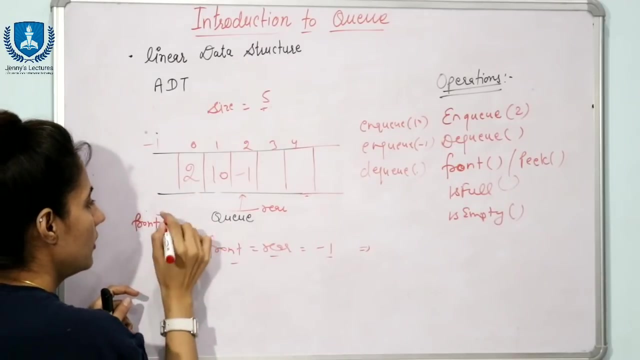 front, right. so now, suppose you want to print the data you have dq'd so you can write down printf. the data you have dq'd is from the queue. you can print this value and after that what you will do, you will do front plus plus, right. so now front is pointing to here. front is one, rear is two. 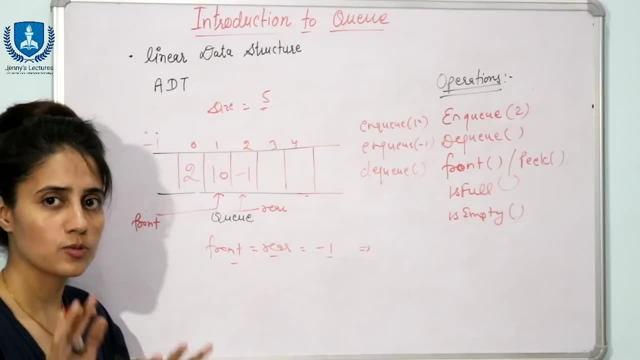 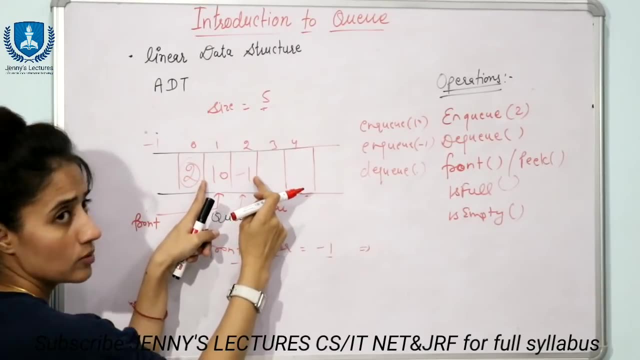 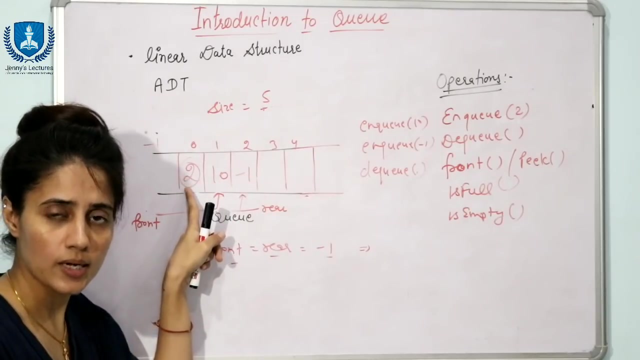 or in dq. simply, you will write front plus plus. that is also fine, because now this is not a part of q. the part of q is only two elements, whatever between front and rear. that is part of q. this is now a garbage value, and we don't care what garbage value lies here. in future, if you will, 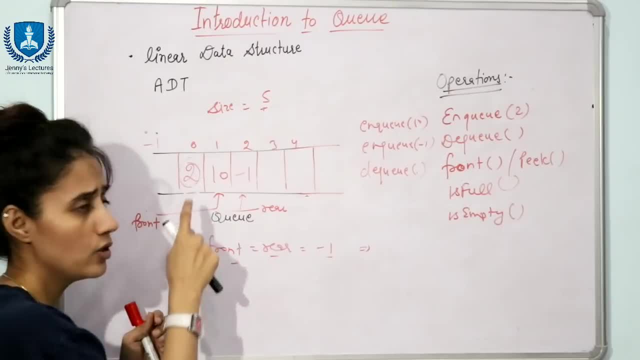 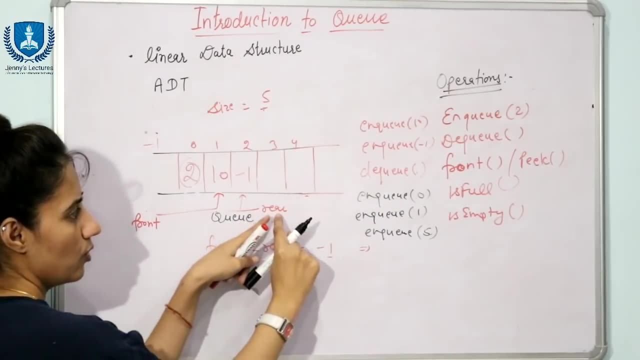 access this cell and if you will write here something, then this value would be overwritten. that is fine. fine, now suppose i am calling nq function three times. so now nq is zero means from rear. i will not touch this front from rear and rear only. i can insert here plus, plus rear. 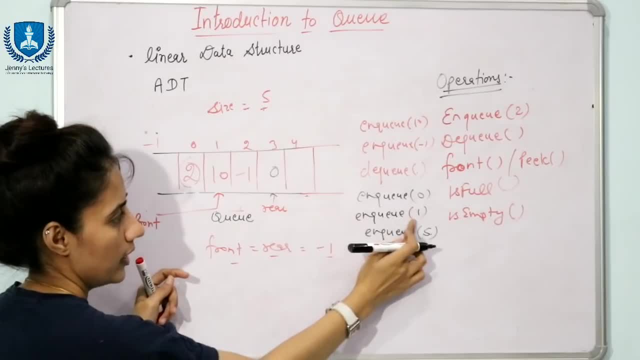 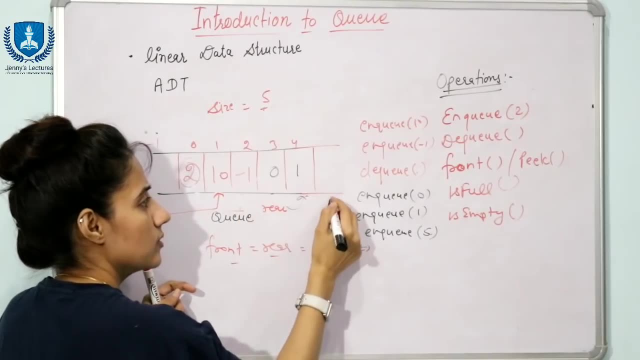 would be pointing to. here and here i can insert this value from rear and rear only i can insert rear plus plus rear, would be pointing to. here and here i can insert here and here i can insert zero nq, one rear plus plus. here i can insert one nq five, then rear plus plus, but what we have, the 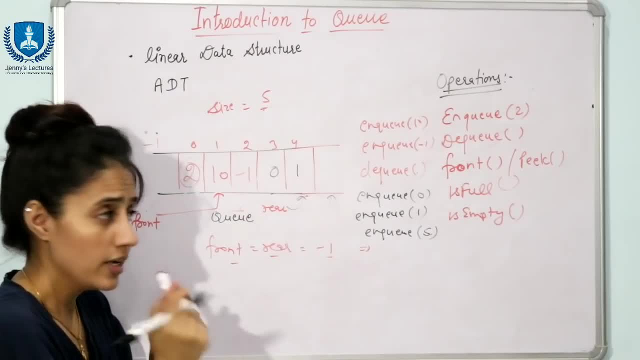 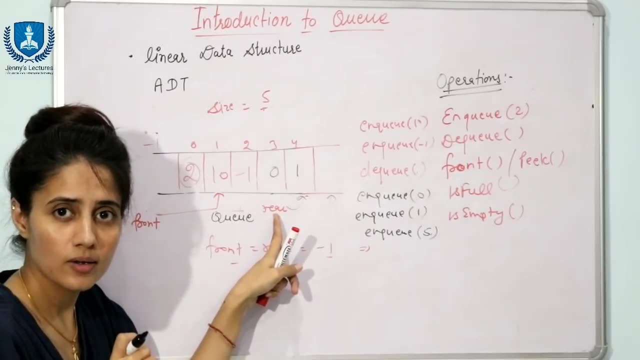 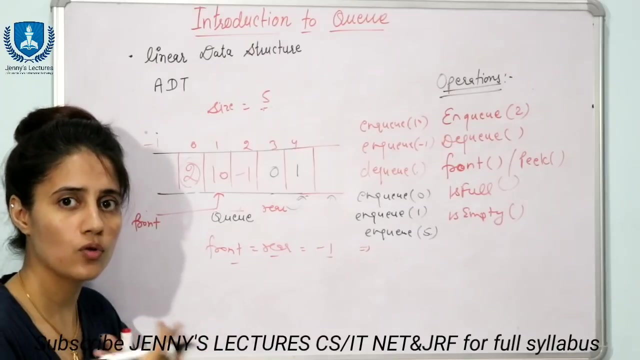 size till here only so if rear is what rear is equal to four, it means rear is equal to this. maximum size minus one index is four. now maximum size is five. in that case you will print. we cannot insert any data. it means you can say overflow condition. this is overflow condition, right. 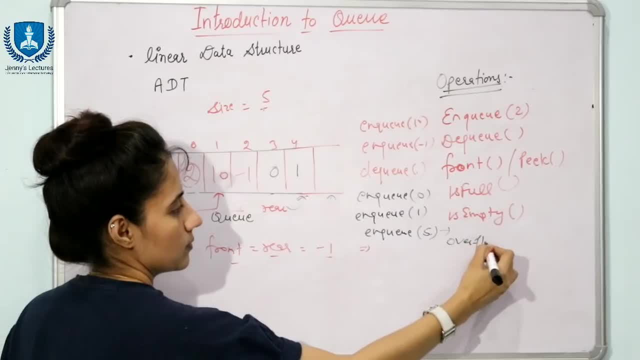 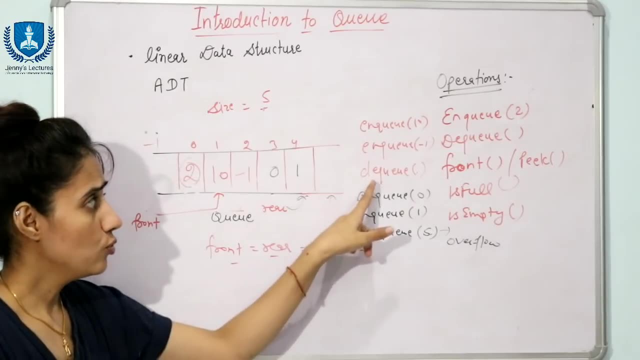 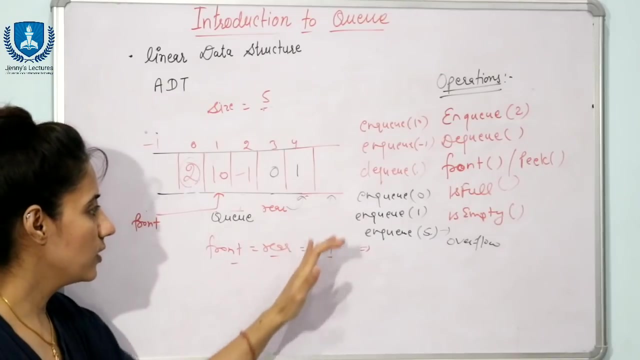 so this would print what overflow condition this is now of overflow condition, right? and what is underflow condition? suppose you want to dq and there is nothing in this list, right, both front and rear are minus one. in that case, what that is an underflow condition, that is q is. 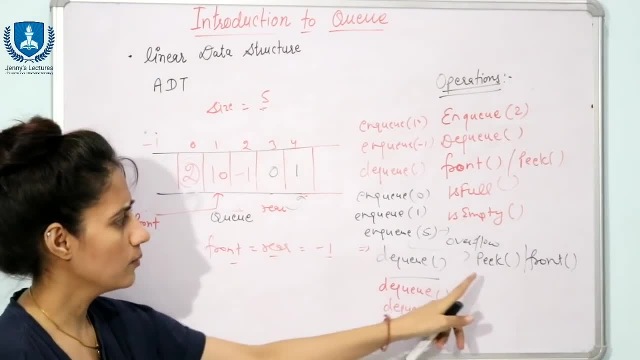 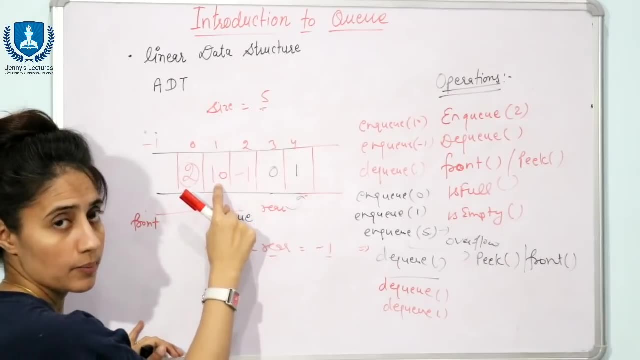 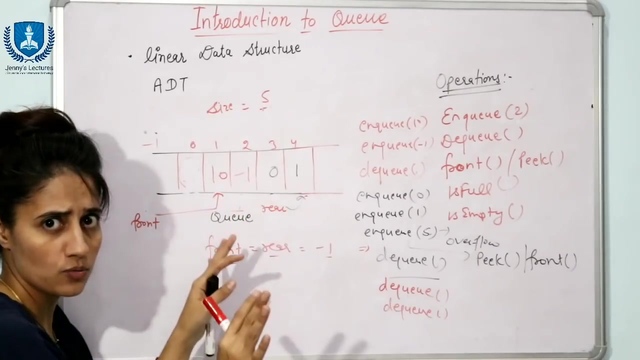 empty right now. suppose, before calling this dq function, i am calling peak function after this nq. or you can say front, so it will return. what front value is now? 10, because see, q is between from front to rear, that is, here to here. this is what garbage value. so i'll rub this one. this is garbage value, right? so now? 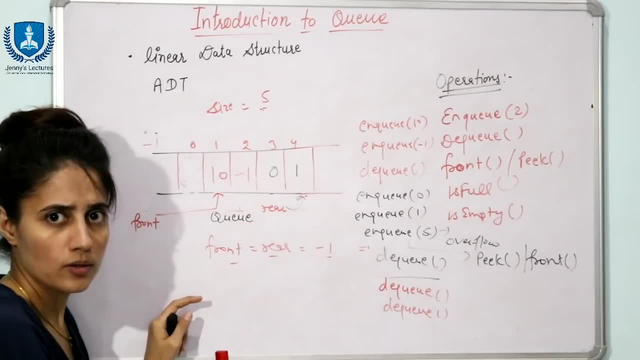 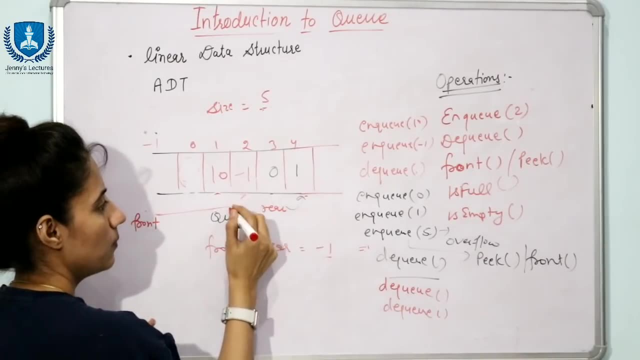 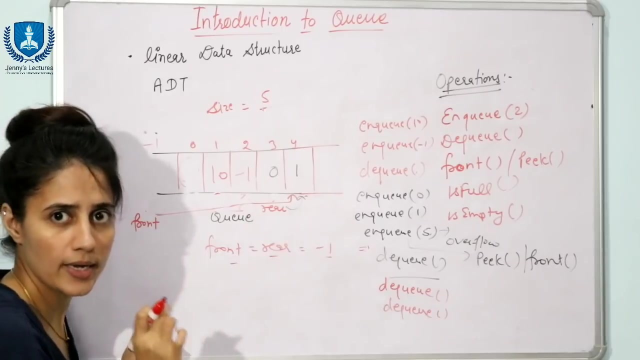 this will return 10.. after that, suppose you are calling dq function continuously three times. what would happen? first of all, dq. it means front plus plus front would point here again. dq. front plus plus again. dq. front plus plus right means front and rear. both are pointing to here now. 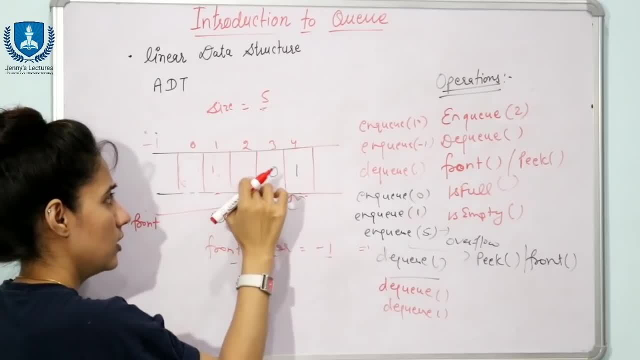 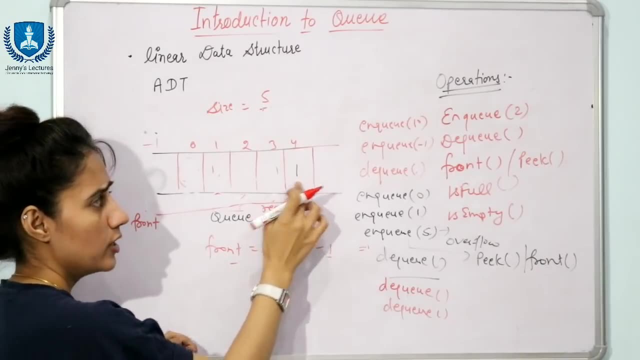 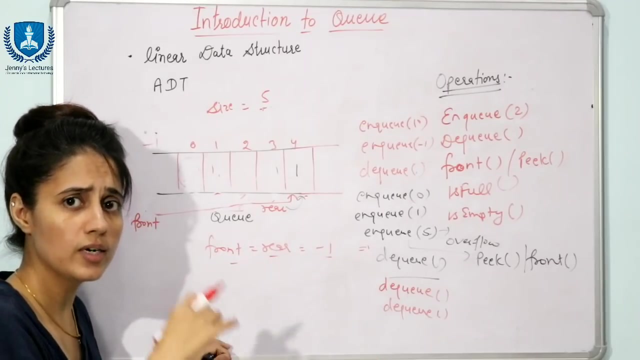 this is what a garbage value. this is not a q. suppose i'm removing these values from here, from these cells, because you can overwrite these values. right now, as you can see, both front and rear are pointing to hair. both are at same index. so in dq you can write down one condition. you can check with that condition also if front and rear is. 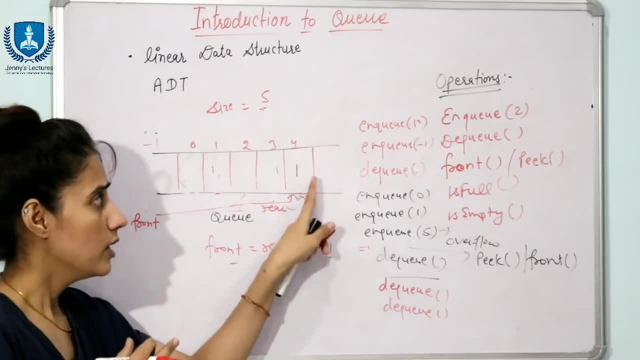 equal if front is equal to is equal to rear. in that case, what it means only one element is there in the queue. so what you can do after removing this, what will? what would happen? front and rear is equal to front and rear is equal to rear. in that case, what it means only one element is there in the queue. so what you can do after removing this, what we? what would happen? front and rear is equal to VS. any value of root correct. q is remaining. 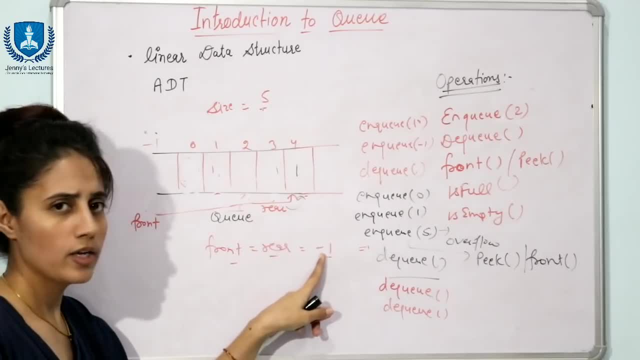 of root contract from we theigon: 27.10관. front and rear is equal to minus one. you can set front and rear is equal to minus one because this is the condition we have set for mptq, right? or if you will not do this thing, 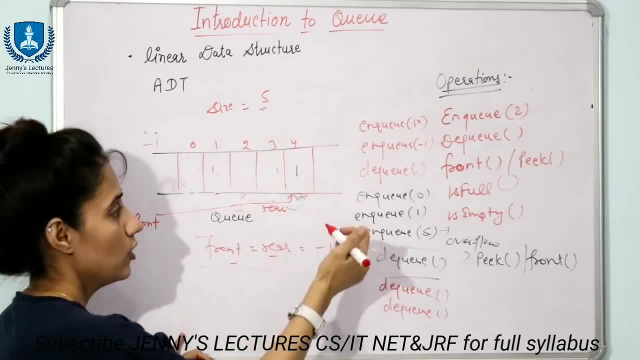 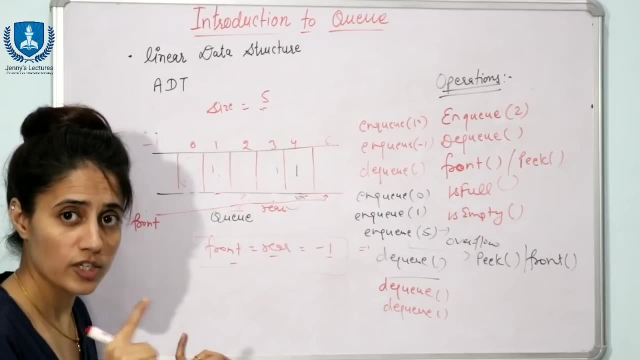 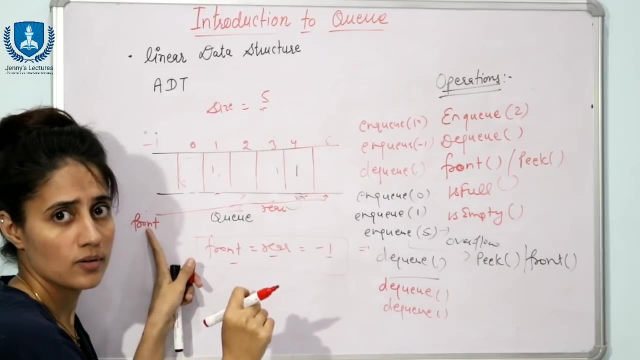 then simply same processor: front plus plus right. front plus plus means front, would point to here that is five, front becomes five. so another condition of checking the mptq is: what if front is greater than this rear? because rear is still four, front is five, right in that case? 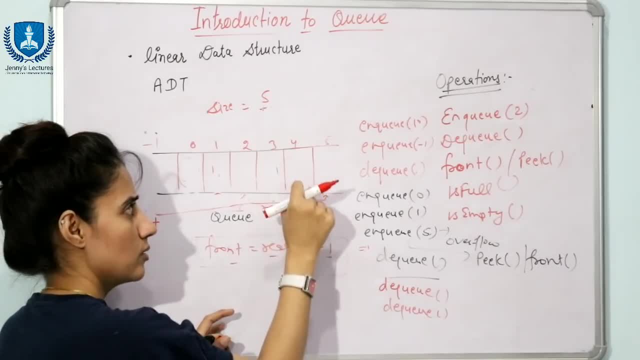 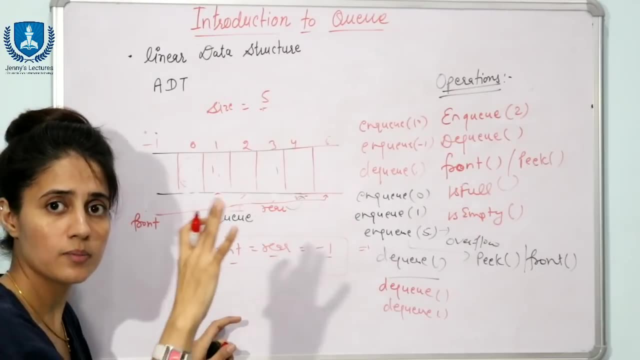 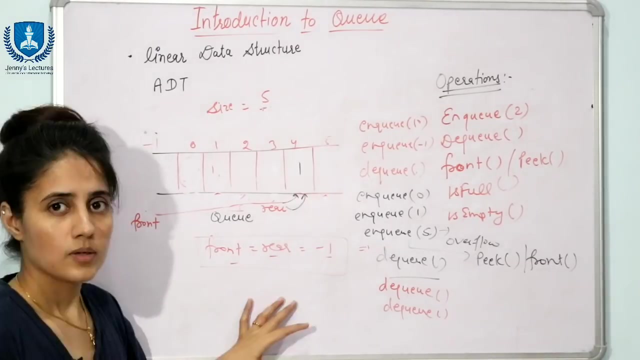 it means q is empty. front plus plus means we have deleted this q, right, so deleted this element from the q. so it means q is empty. so when front becomes greater than rear, then also it is empty. so we are going to see how to write down these condition in next video. fine, now suppose. 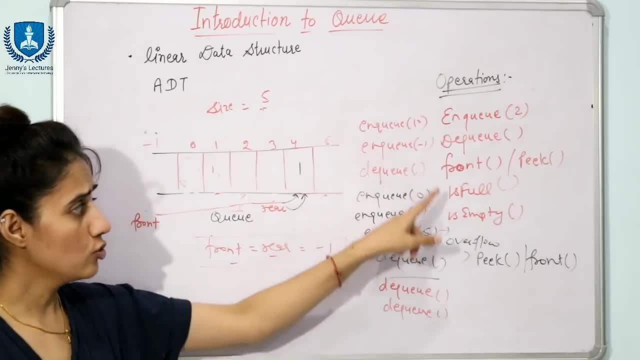 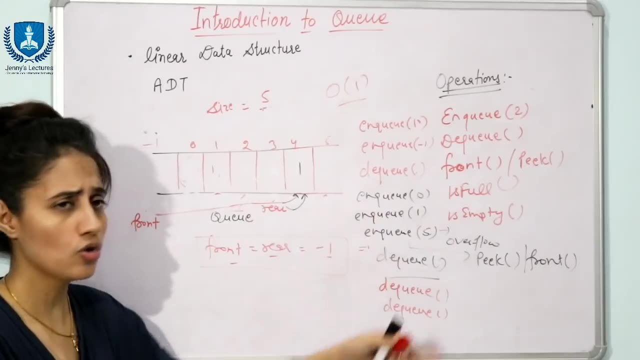 if you talk about the time complexity, then in that case these operations would take order of one and two. so we are going to see how to write down these conditions in next video. fine, now, only because we are not going to write any loops or anything for performing these operations. so it 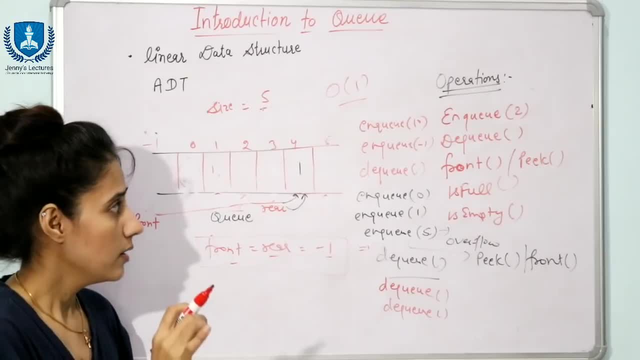 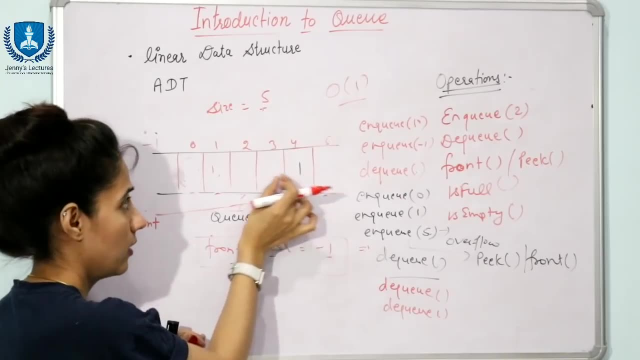 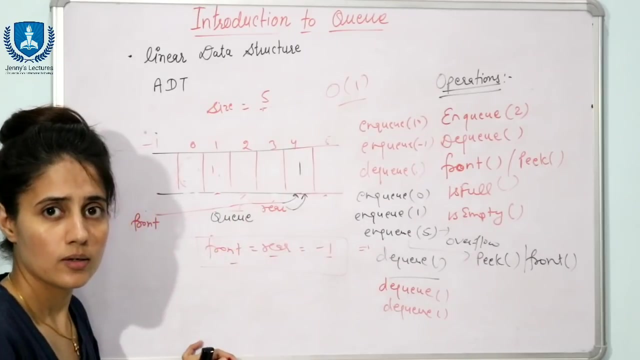 would take order of one only right, constant time. now suppose at some point of time both front and rear are pointing to this node. it means q is having only one data: this, this, this, this. these four cells are empty, right and now. if you call nq, in that case it would return what q is full. 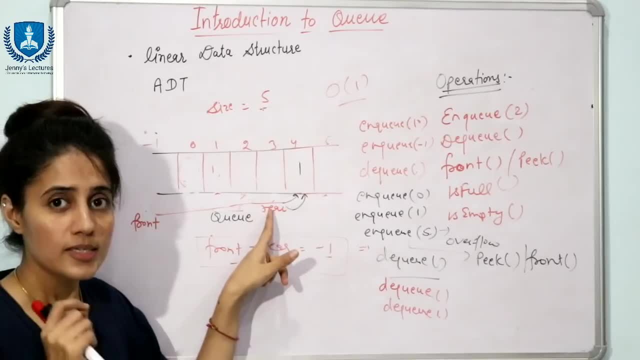 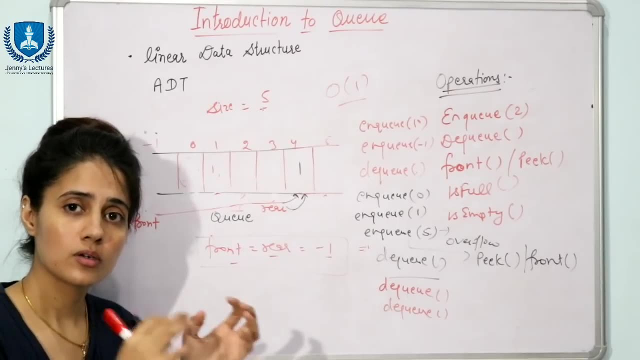 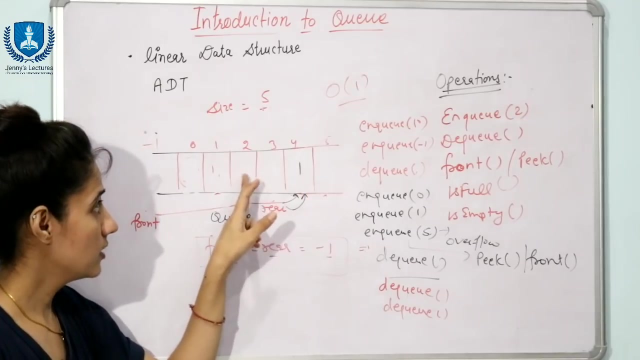 that is the drawback why it will return. q is full because, see, see, here here is what pointing to four. here is four, that is maximum size minus one, and that is condition of what overflow condition means the q is full. now it will show you q is full, right, but see, these spaces are free, but we cannot insert here this. 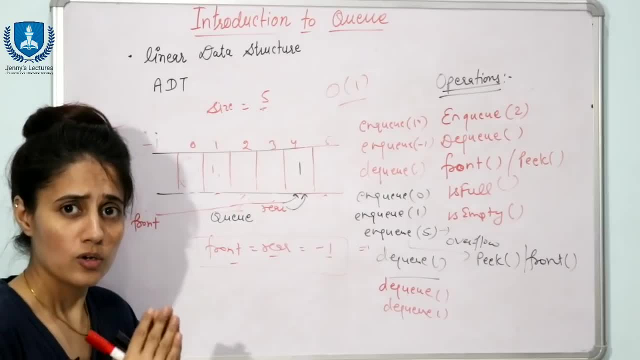 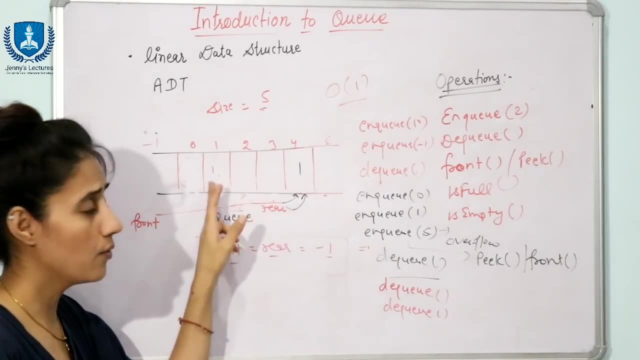 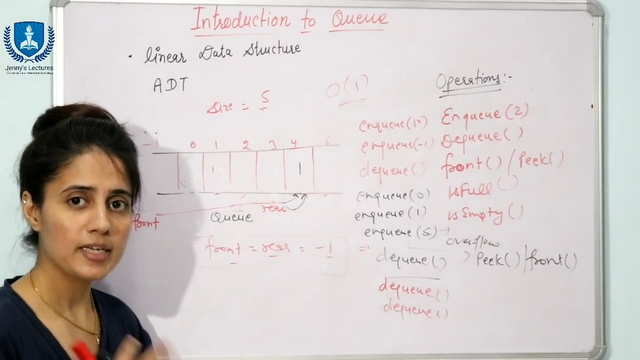 is what wastage of the space. so this is drawback of this q. we have a solution of this q, that is, the circular q. that also we will discuss later. fine so, but this is now a drawback. you have space, but you cannot insert here data right now. we will see some applications of q. 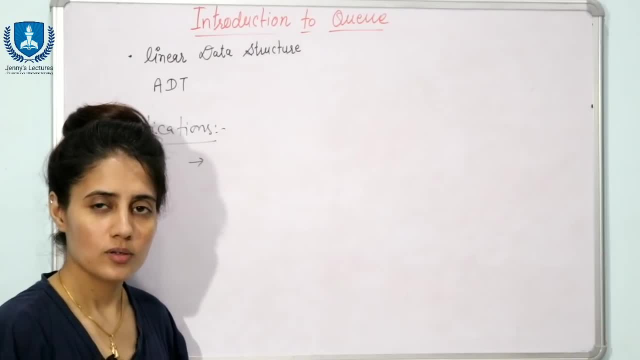 so the most common application of this q data structure is what it is used, where you want to, you know, serve the request on a single shared resource. suppose you have a single resource and that is shareable. let us take you- you can take an example- of printer. suppose you have one printer. 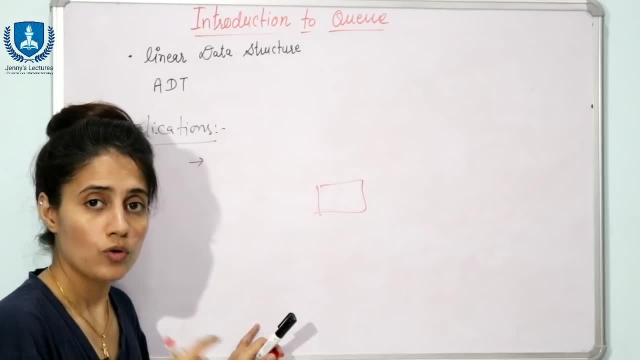 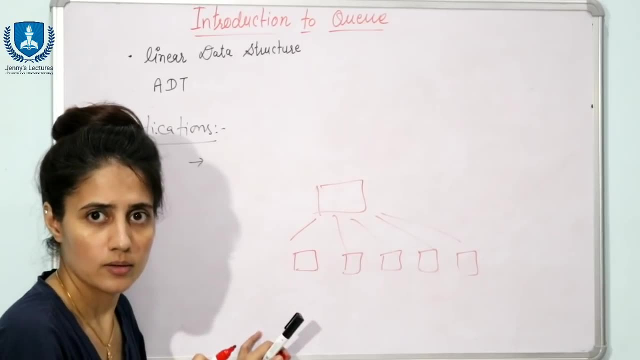 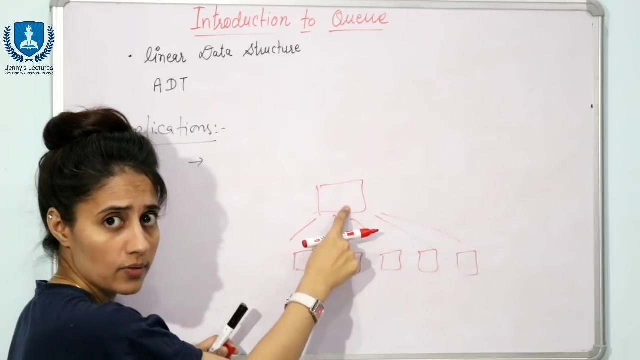 and that is shareable. fine. so what would happen? it is not like that. suppose there are five pcs and these five pcs are sharing one printer. it is not like that: it will give command and this will print and at the same time it will print. it will give command and it will print. right, what this printer will do. suppose 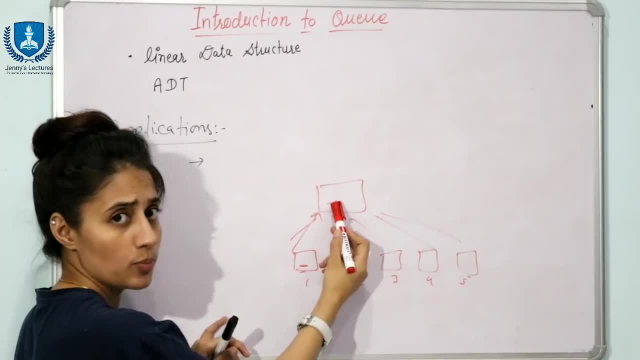 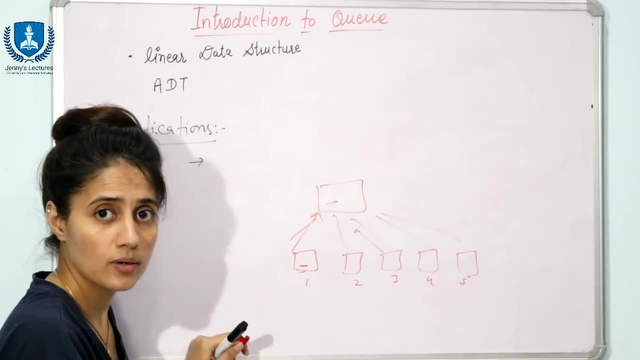 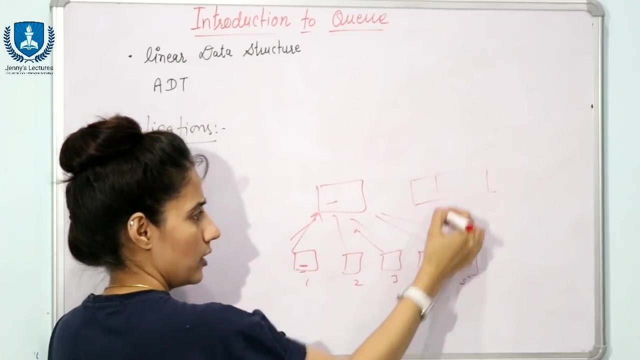 this. this has given some command to printer data and now the printer is printing now at the same time computer this three. it has given command to this printer. then what would happen? the printer is busy now, so what printer will do? it will, obviously it will have a program. so that request. 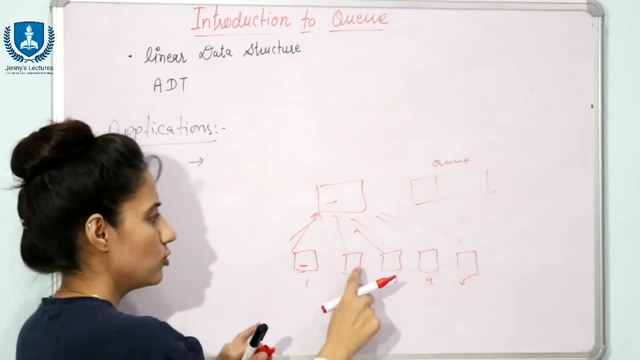 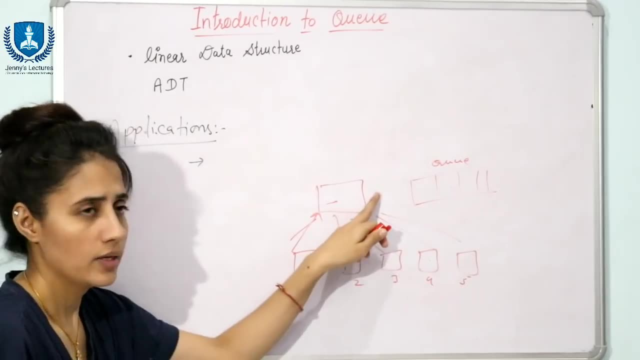 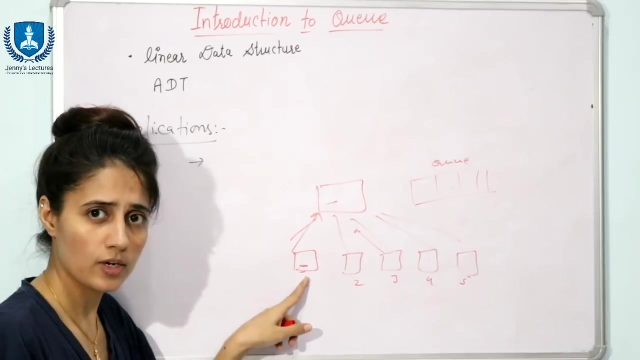 would be stored in q after that. suppose this printer would give the request, so it would store here. after that, this this would store here, so it will in the memory, in the printer memory. it will what make a queue of all the request right? first of all, it will print whatever the request it has. 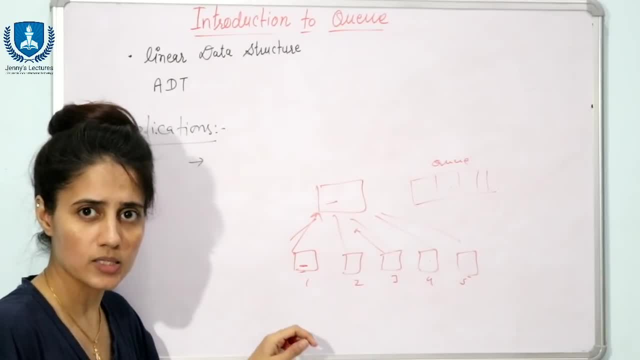 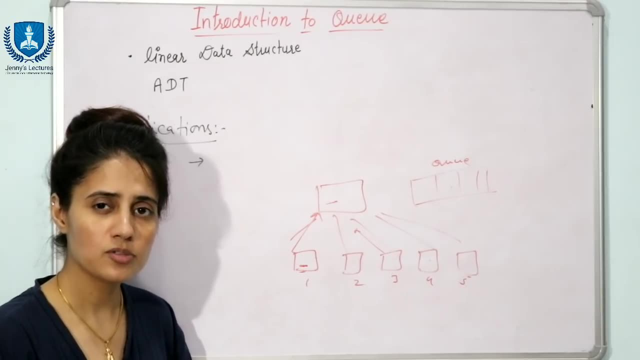 given, then it will fulfill request of three, then two. like this right and queues are also used in real life scenario, like you can take an example of when you call in customer care, then sometimes they tell you that they tell you to hold on for few minutes because their representative is. 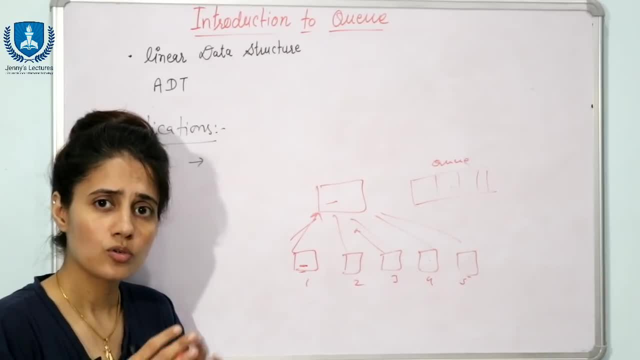 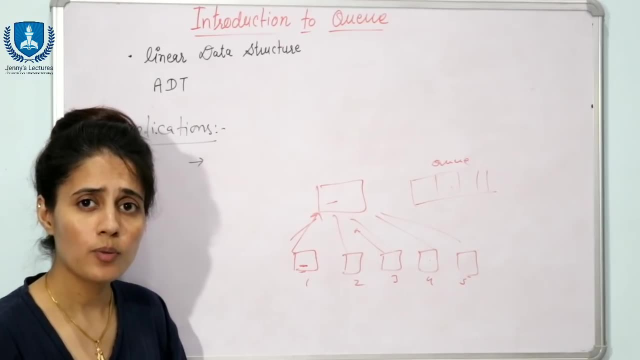 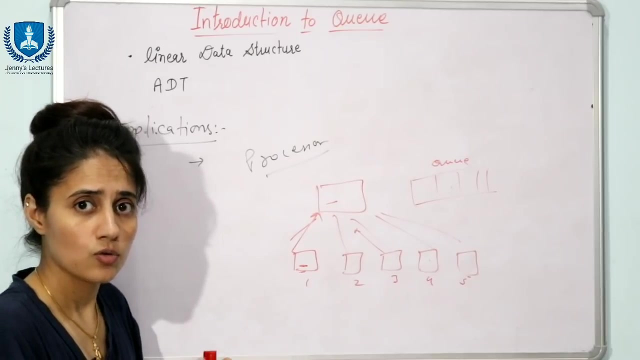 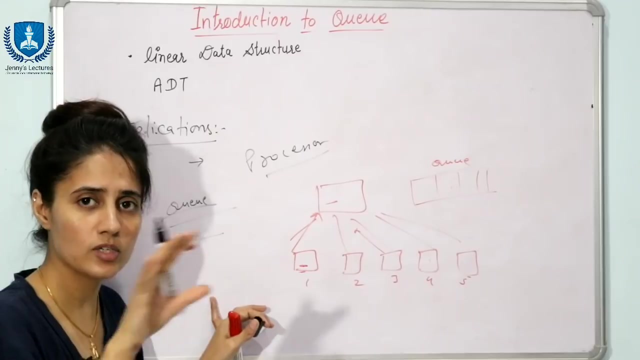 not free. so what they do? they use queues to put the people on hold right until their representative are free. fine, next you can take an example of processor. see, you have only one processor CPU, you can see. right, so the processes would be placed in queue in operating system. I guess we have discussed many times, when we were discussing the concept of 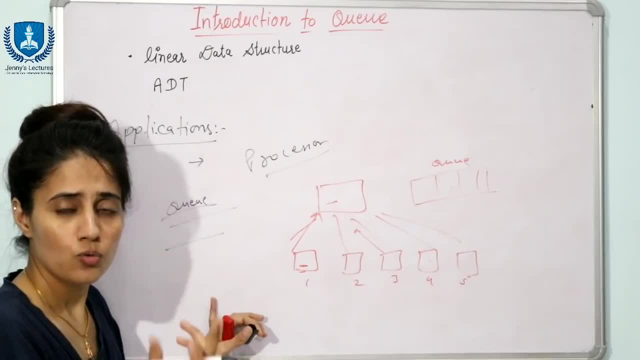 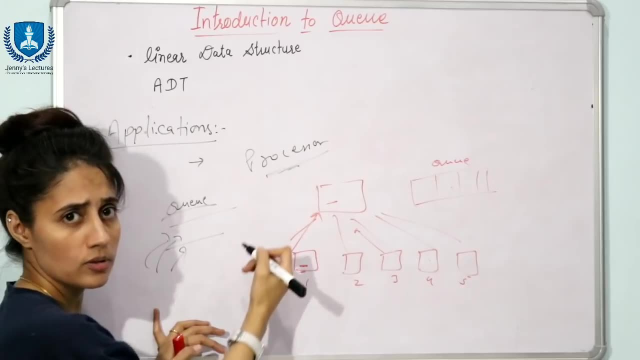 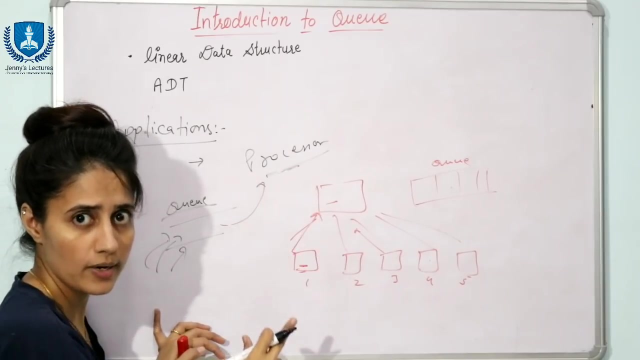 operating system. then you can check out in the playlist. there are ready queue, there are waiting queue- fine, so the processes would be put in the queue and as soon as processor gets free it will take from the queue. it will take the processes from the queue one by one right. so all the